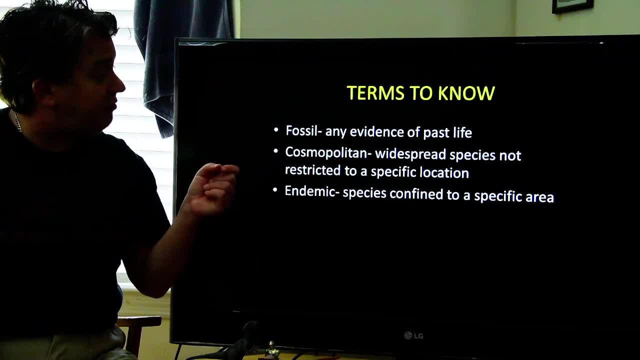 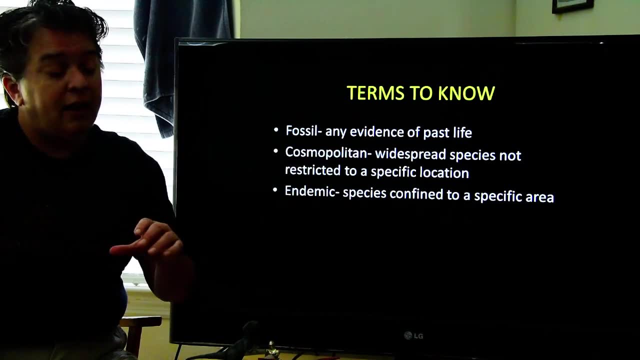 Now here are some terms to know as we start studying fossils. Well, today when we use the term fossil, it means any evidence of past life, And it didn't always mean that If we go back in time to like the Renaissance or the Middle Ages. 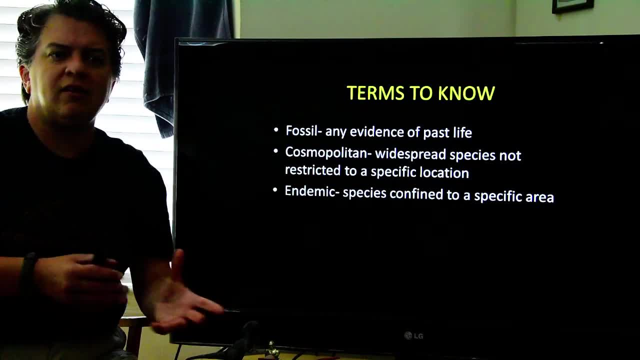 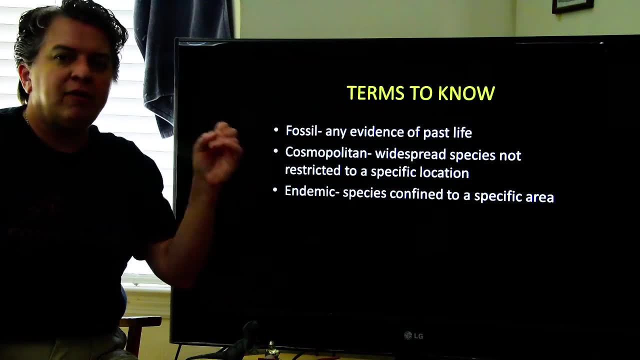 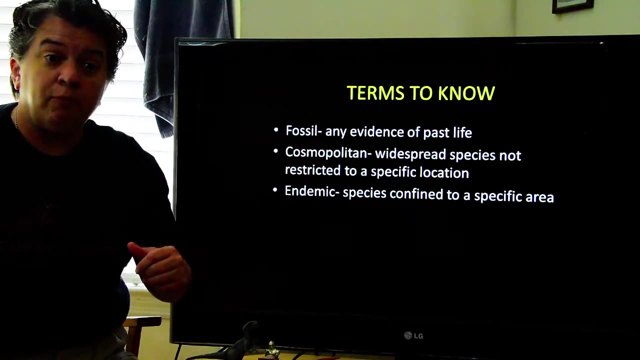 fossil referred to anything neat that you would dig out of the ground, anything that had a weird shape or looked cool. But today it means evidence of past life, And when we describe organisms that are alive today or were alive in the past, we might use the term cosmopolitan. 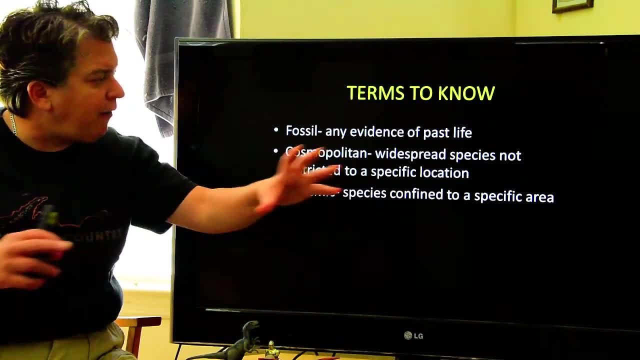 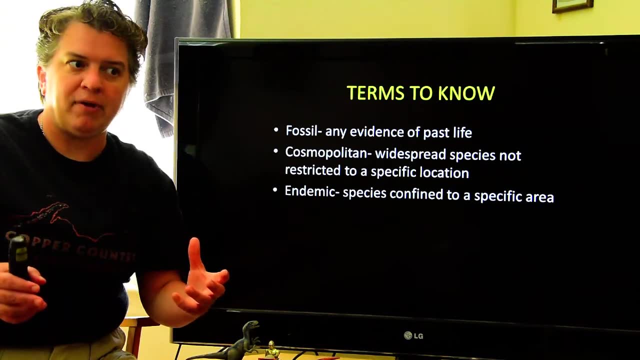 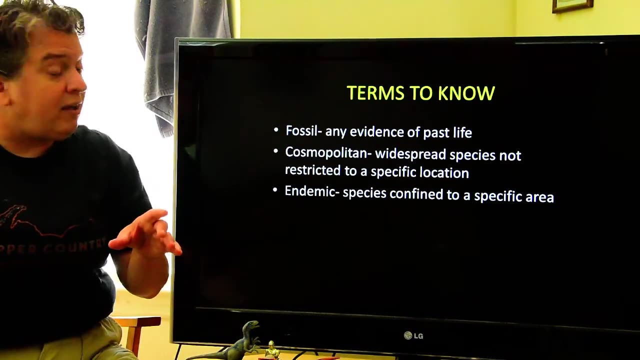 This means we're talking about a species that's very widespread and not restricted to a specific location, So you could say that a homo- sapiens. our species is very cosmopolitan, right? We live all over the world For organisms that are not that way. 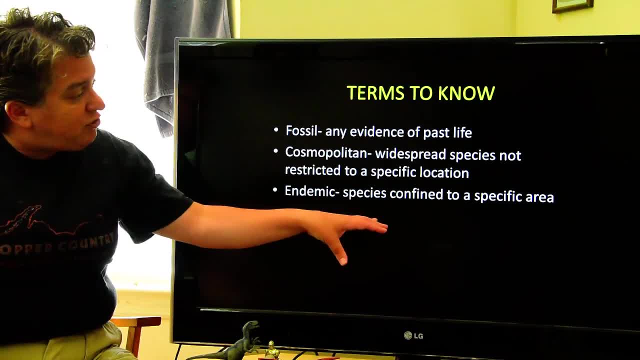 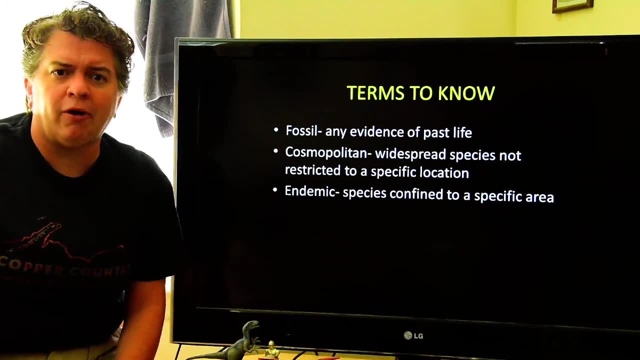 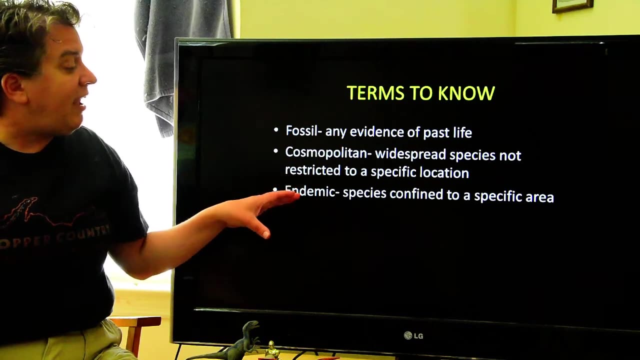 we use the term endemic And this is species that's confined to a very specific area. So, for example, there's a certain type of bird that only lives in the Galapagos Islands And well, we would say that bird is endemic. 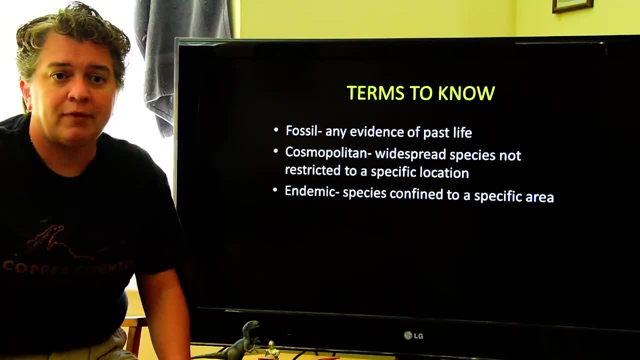 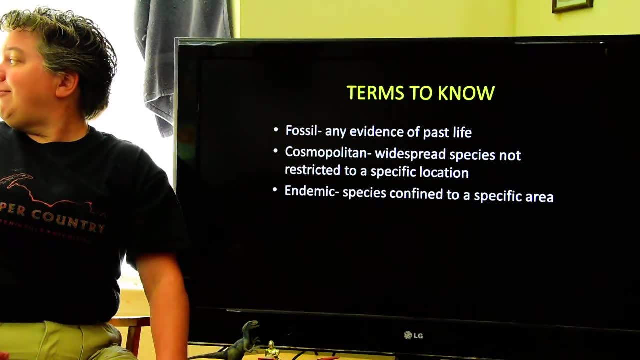 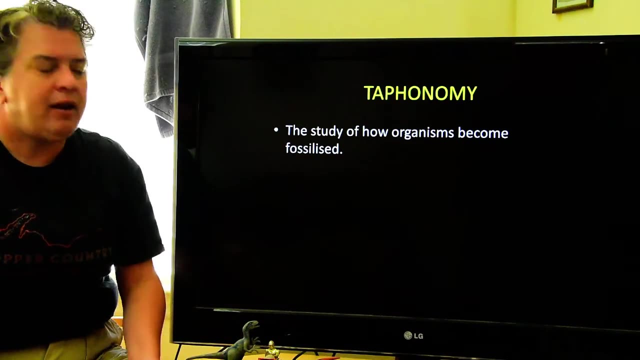 to those islands. It's limited to those, And my cat has allergies, so you probably hear the poor little guy sneezing You. okay, little fella. Okay, Alright. now when we study how fossils are created, this is called: 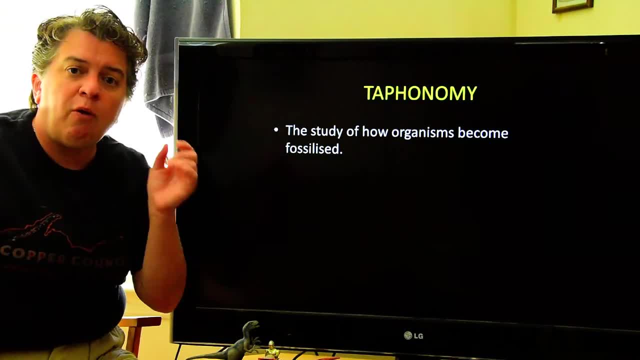 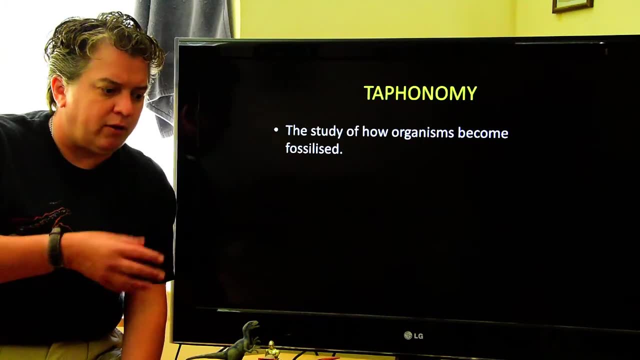 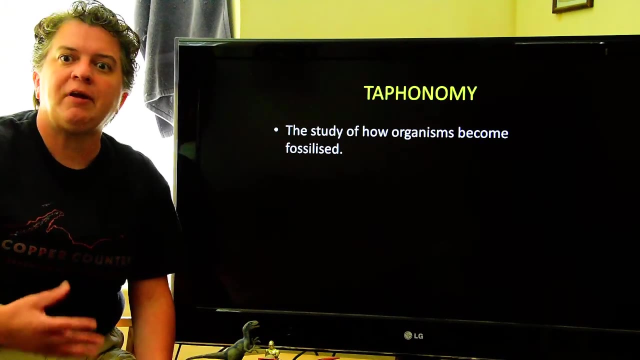 taphonomy. Taphonomy is the study of how organisms become fossilized, And it's something you can actually specialize in. You can look at, Well, when a shelled organism dies, how does that shell end up getting preserved for us? 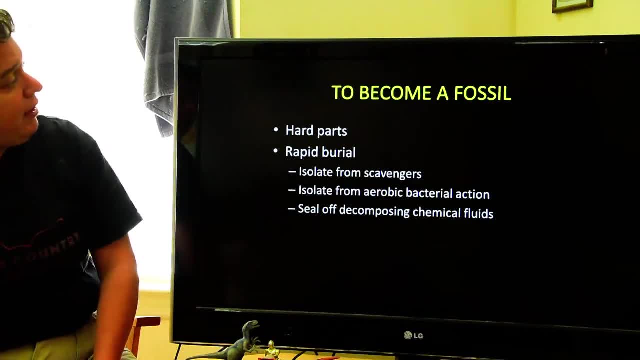 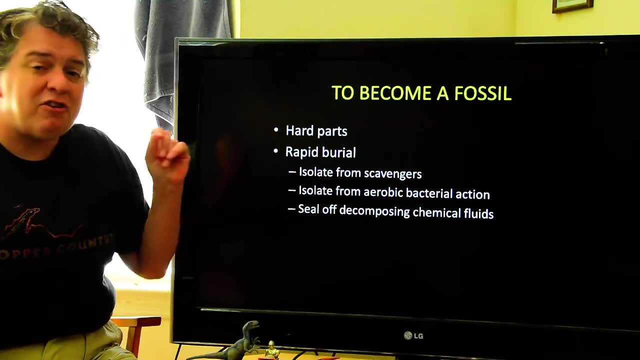 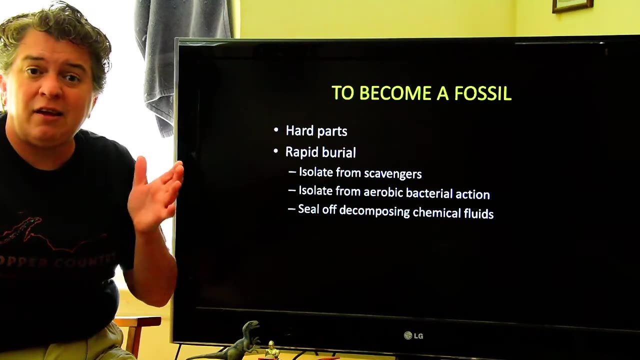 to then see millions of years later. Well, there's a few things that help organisms become a fossil Possession of hard parts. If something is just soft and squishy, like a jellyfish or so, it's not as easy to preserve. 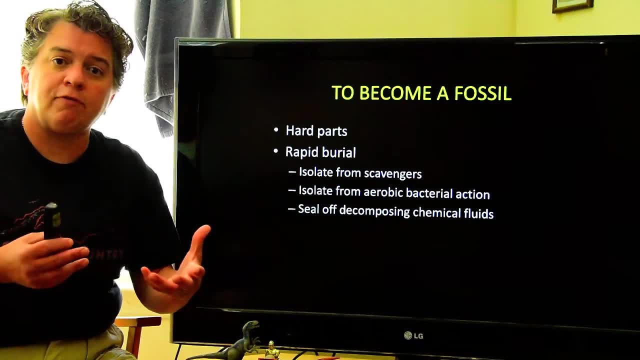 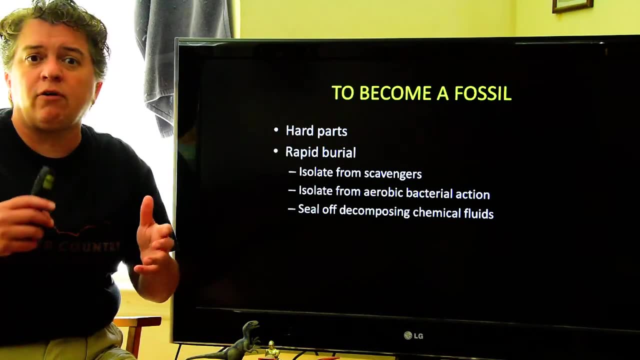 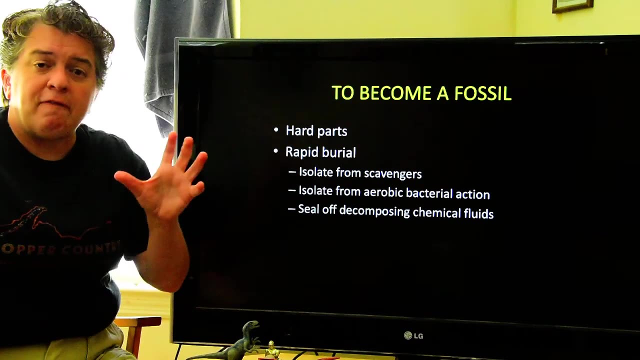 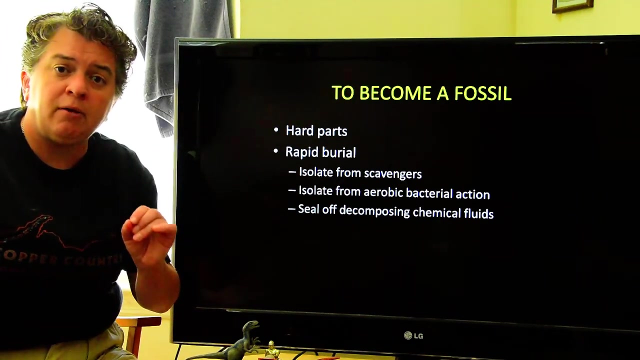 I'm not saying they can't be preserved, but it's harder for something that's just soft and squishy to be preserved. So having hard parts like a shell or bones or teeth really helps. Also, rapid burial: The faster that this deceased organism can get buried, the better its chances of being. 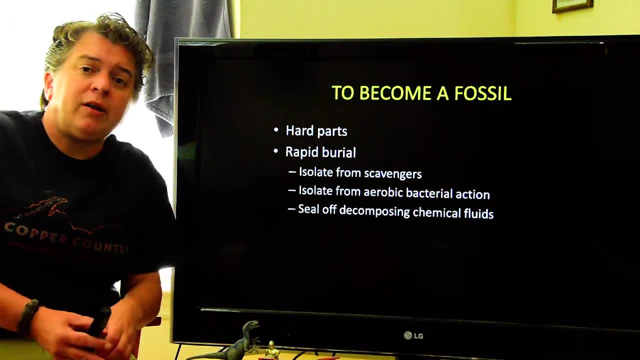 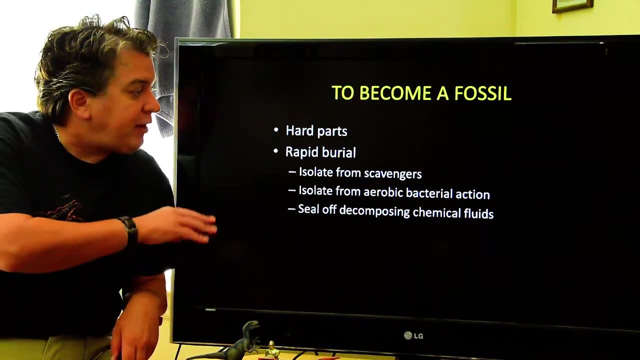 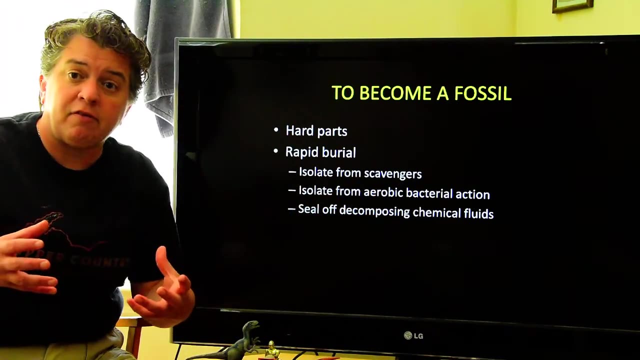 preserved as a fossil In rapid burial. what it does is it isolates itself. It's isolated from scavengers, so you don't get things like buzzards picking the thing apart. You isolate it from aerobic bacteria, And aerobic bacteria aerobic means. in the presence of oxygen, these bacteria decay. the. 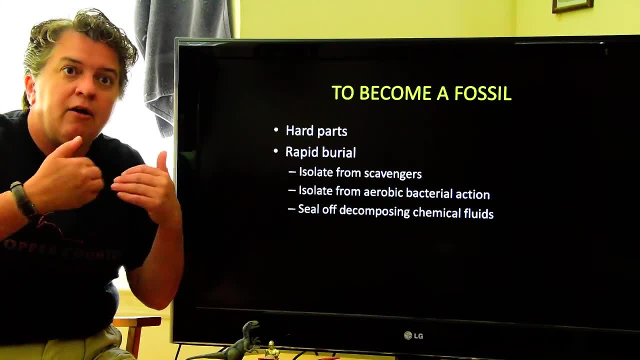 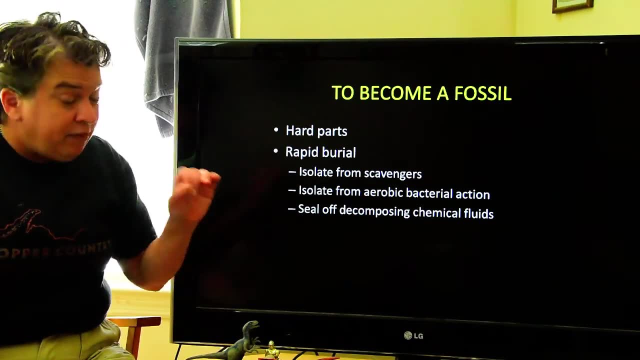 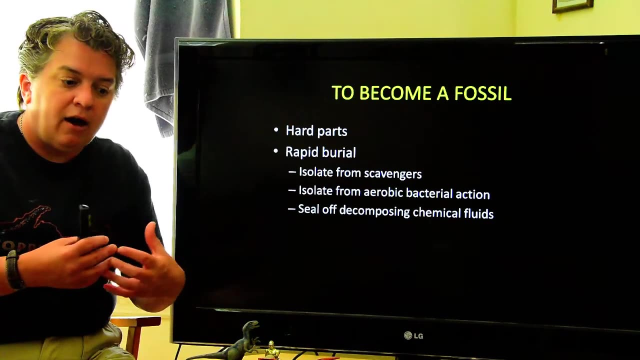 organism And if we bury it, we basically then remove it from those bacteria that will try to decay. that And, in this rapid burial, the sediment that has been buried, the sediment that has been buried that might seal off the organism from chemical fluids that would help decompose. 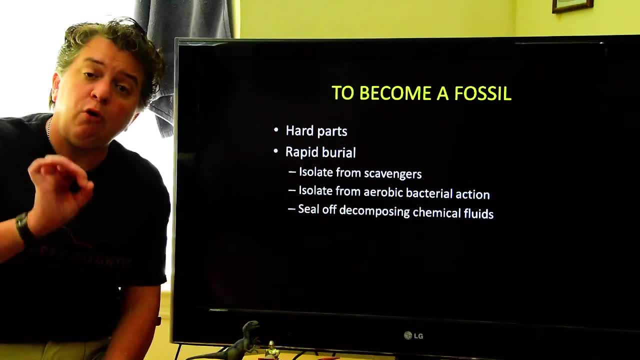 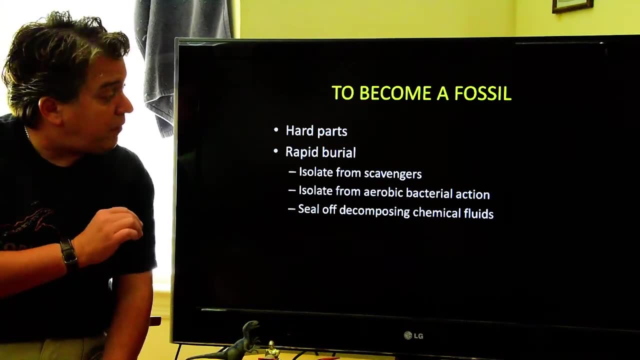 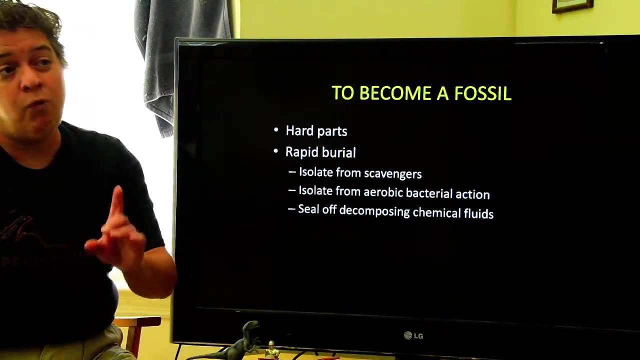 the organic matter as well. So the two big things to help something become a fossil is having hard parts and rapid burial. Now soft tissues can get preserved but, like I said, it's not as common. One thing I would like to add. 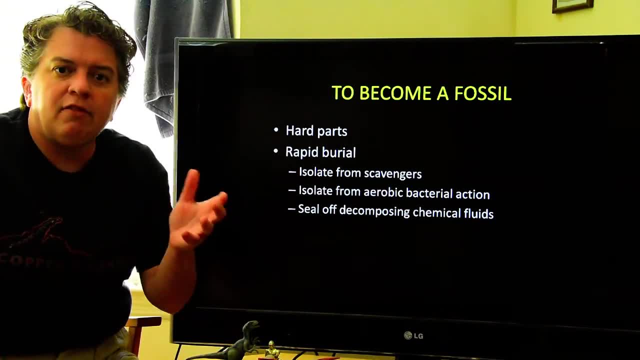 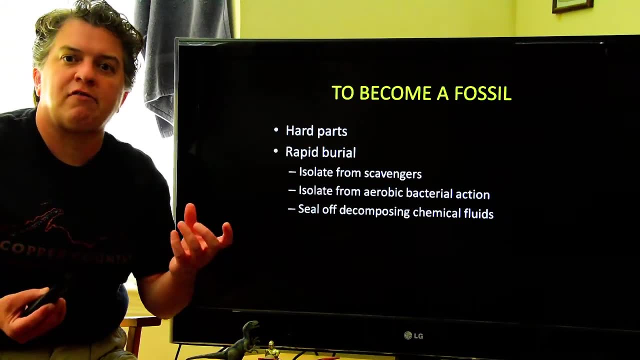 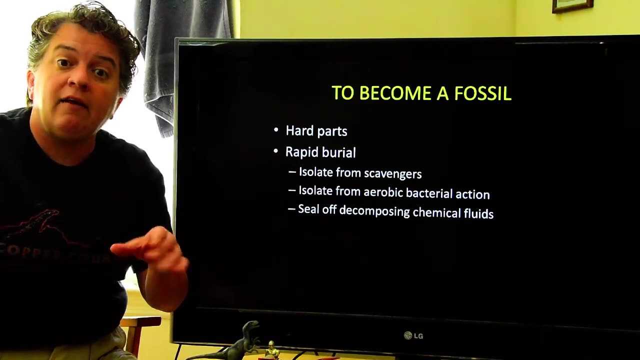 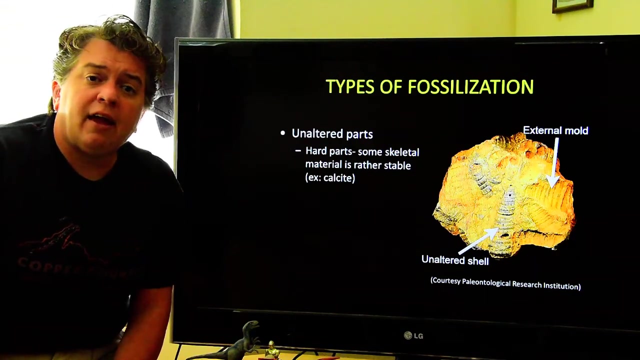 The finer grained the sediment that is burying the fossil typically, the more exquisite the preservation. So really fine grained sediments can preserve lots and lots of detail in the fossils that get buried. All right, so let's look at some of the types of fossilization that can occur. 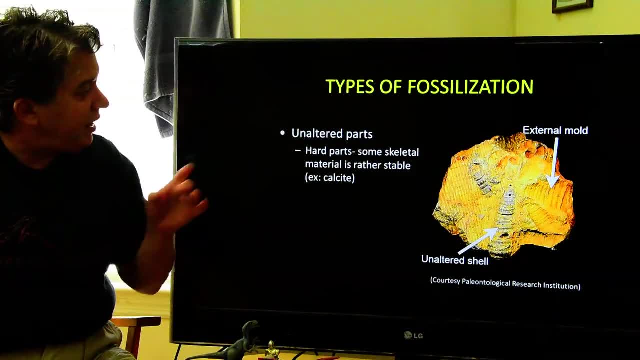 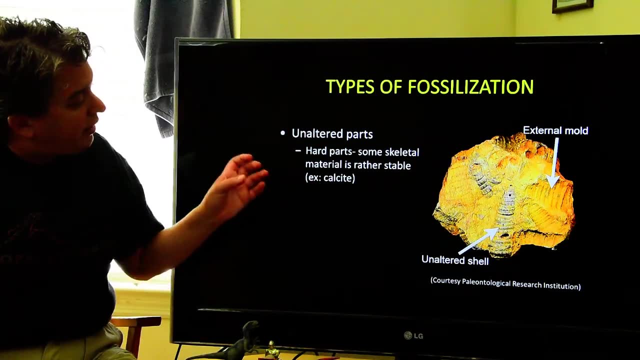 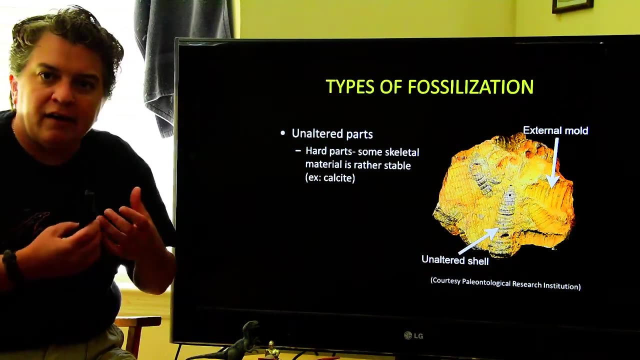 You can have unaltered parts And in hard parts, well, some skeletal material is quite stable, And a great example is calcite. There are many organisms that have created shells out of calcite. Calcite is an extremely stable mineral over time. 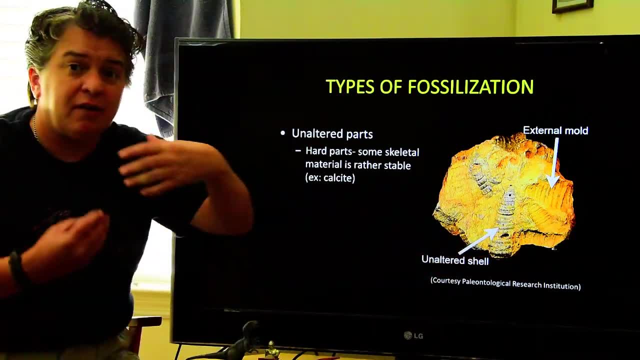 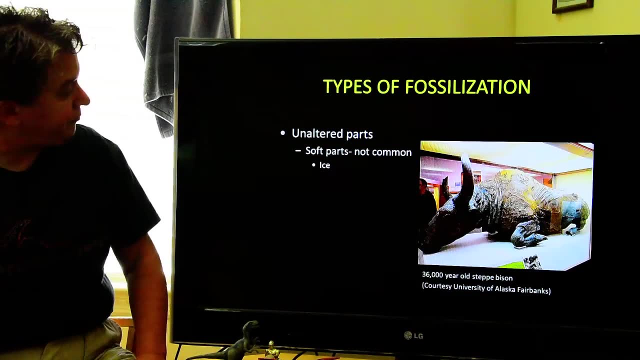 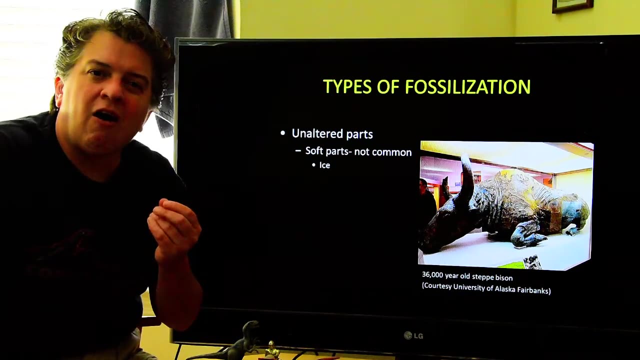 And so you'll have these shells made from calcite, and that's exactly the substance that they were when that organism was alive, So that's unaltered. Now you can get unaltered soft parts, but that's a lot harder to preserve. 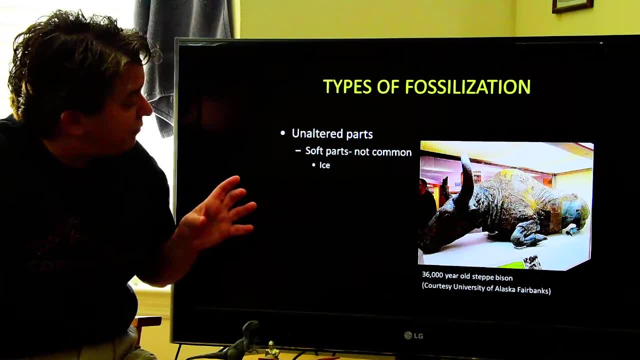 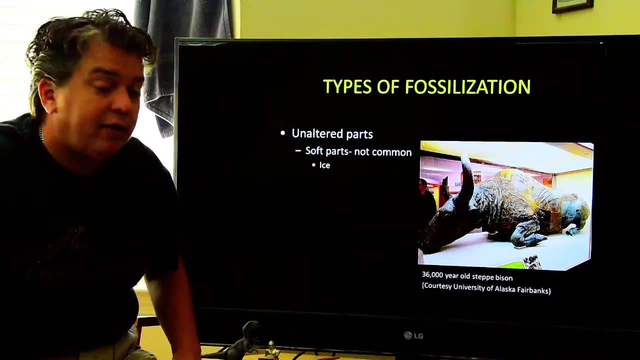 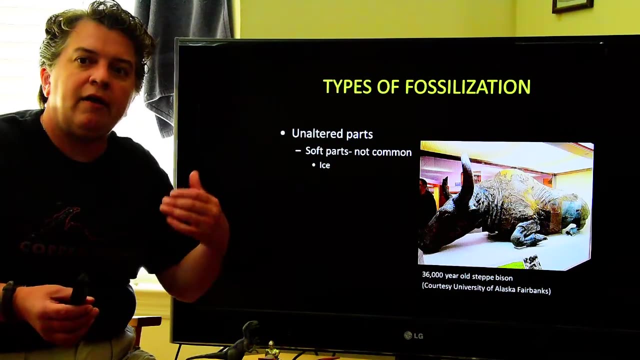 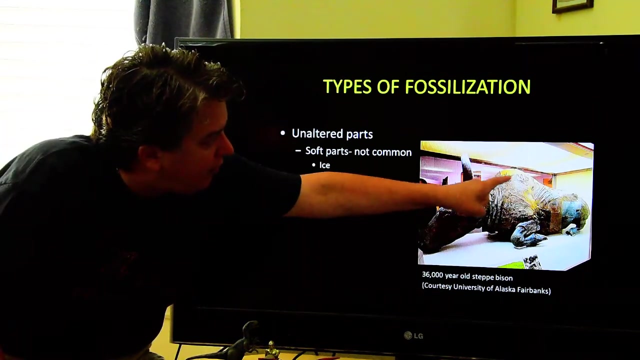 So you might get an ice preserving soft parts And, for example, this is a 36,000-year-old step bison that was trapped in permafrost. Basically, it had fallen in somewhere in the Arctic And permafrost Ice surrounded this organism and preserved it, so you can still see the skin and the hair. 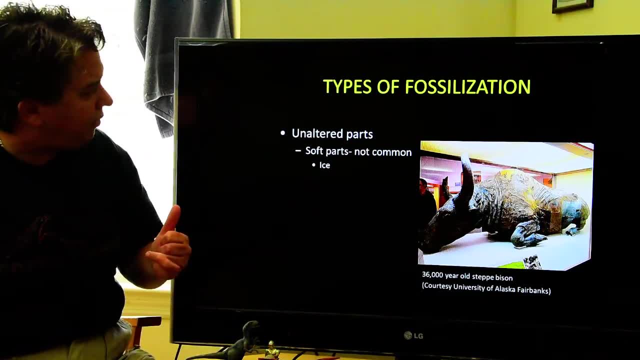 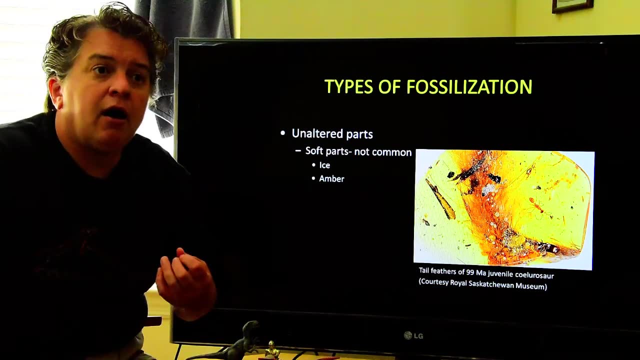 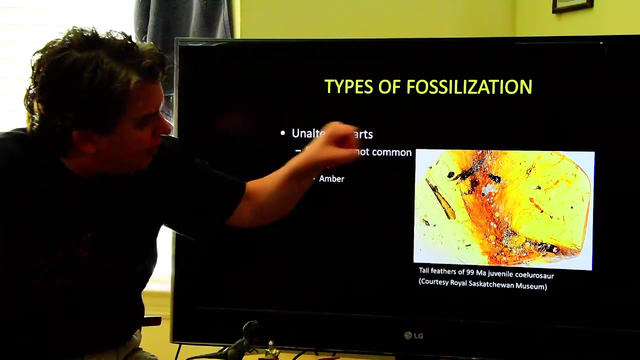 and things on there, And so ice can preserve soft parts. Amber can as well. What we're looking at here, amber is fossilized tree sap, basically, And see this thing right in there. That is the tail feathers of a juvenile silurosaur, which might not mean much for you. 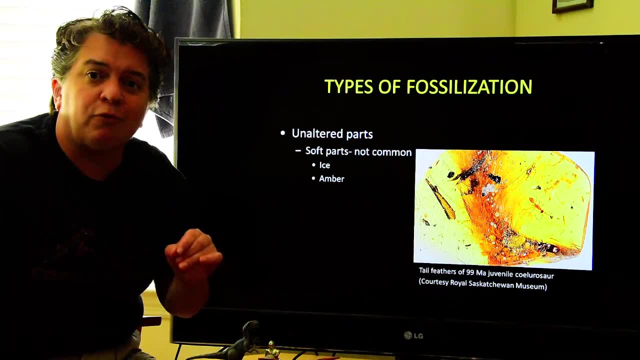 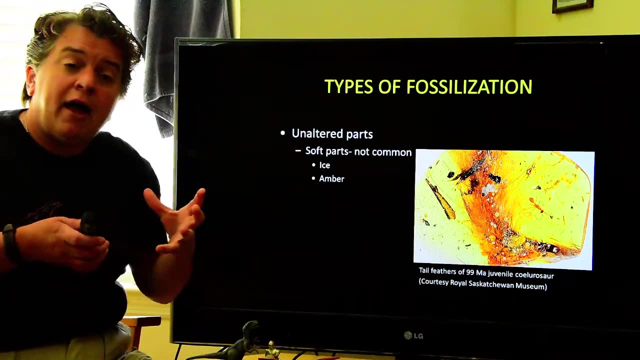 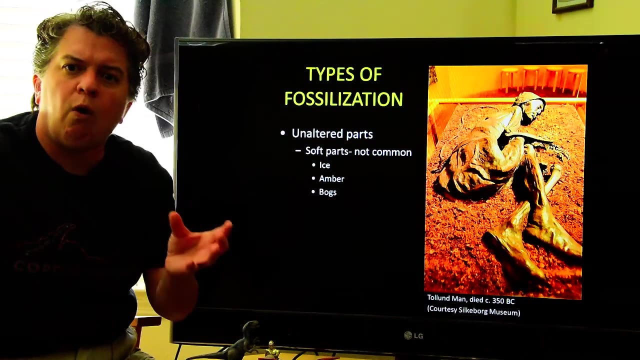 But that's the group of dinosaurs. that includes raptors. So what you're seeing right, there is a raptor feather And we also have an ant, But in any case, amber can preserve these soft parts And then in bogs- because you have stagnant water- you can get soft parts being preserved. 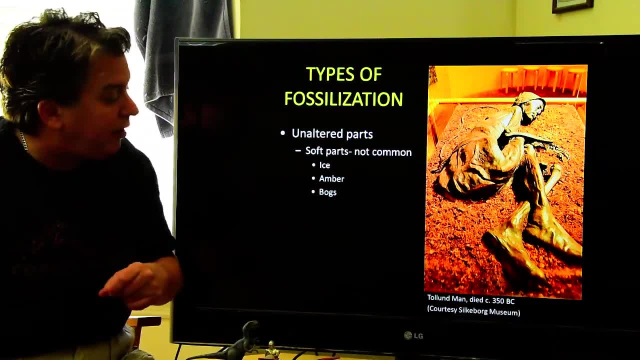 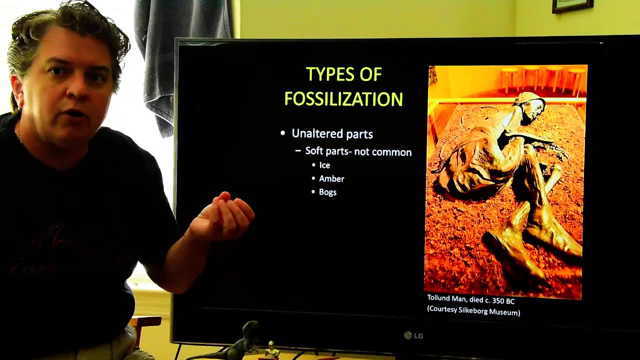 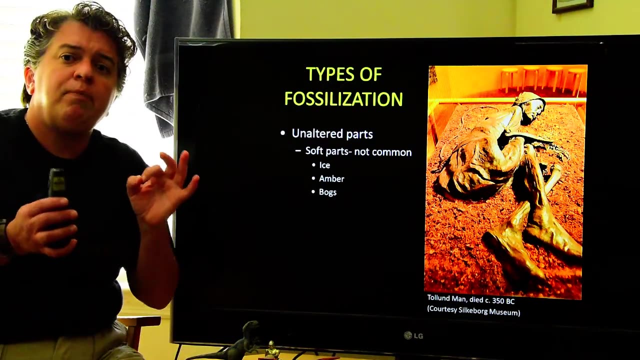 as well as we see in Tallundban here. He died around 350 BC, But the preservation is still so good that you can actually see like the hair on his chin and stuff. So you can get soft parts being preserved. but you do need special circumstances for 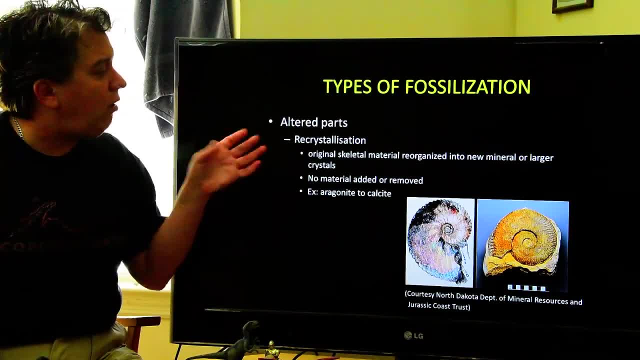 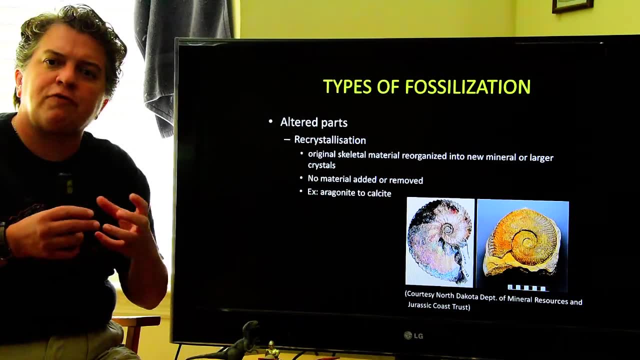 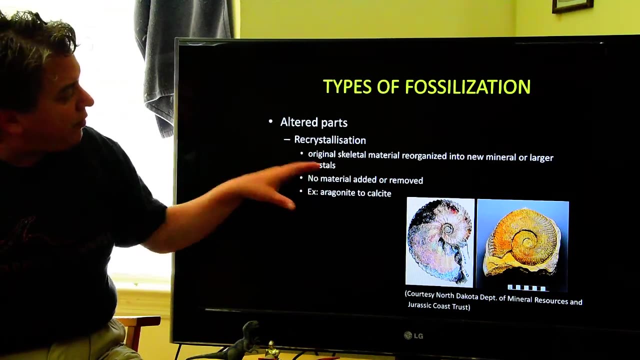 that All right. Now we can also have altered parts, And that means that the fossil somehow has changed from its original composition. So, for example, you can have recrystallization occur, So you can have a fossil, And in this case the original skeletal material gets changed into a new mineral or maybe larger. 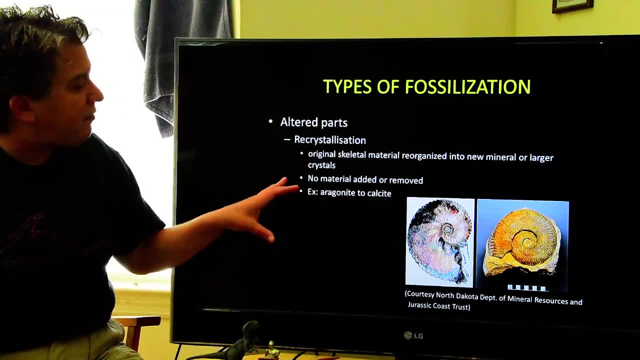 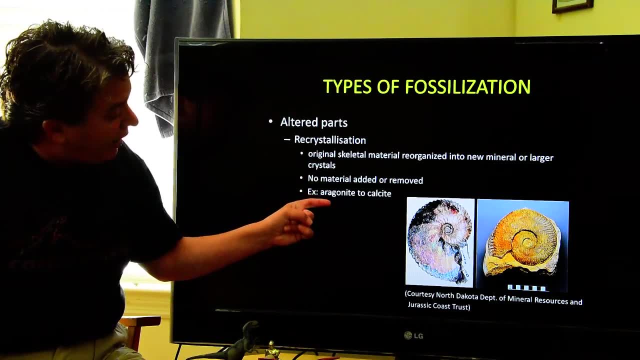 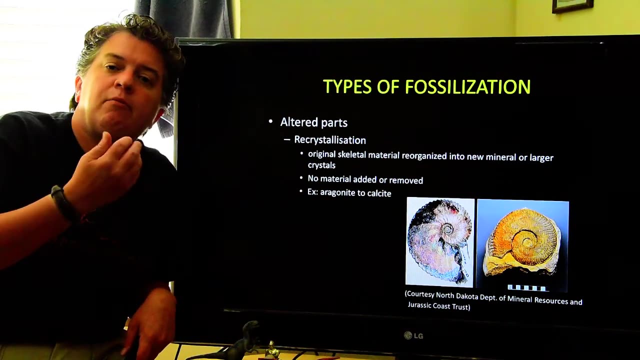 crystals of some kind, And in this case no material is added or removed, And the example is aragonite to calcite. So both aragonite and calcite are calcium carbonate, And so they have exactly the same chemical composition, But they have a different composition. 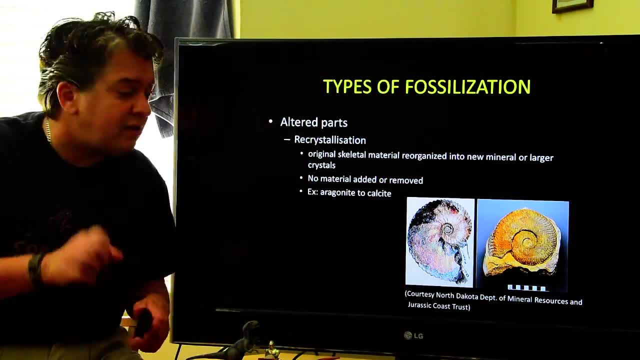 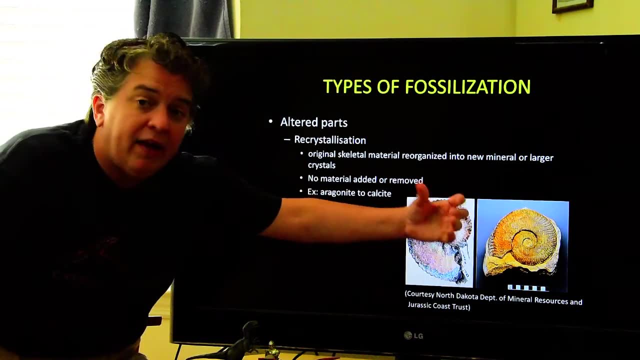 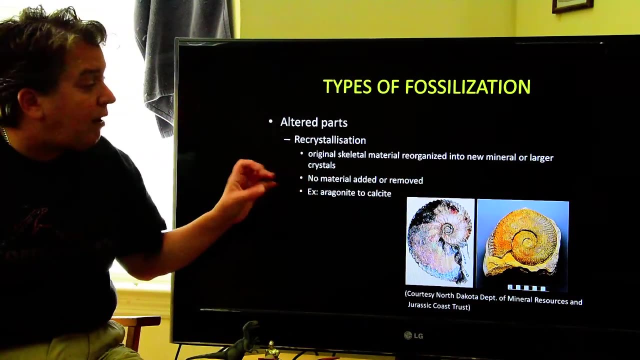 It's just the crystal structure is a little bit different. So you might have an organism that originally had an aragonite shell. well, that shell material will recrystallize into the more stable calcite, And so that would be an example of this recrystallization. 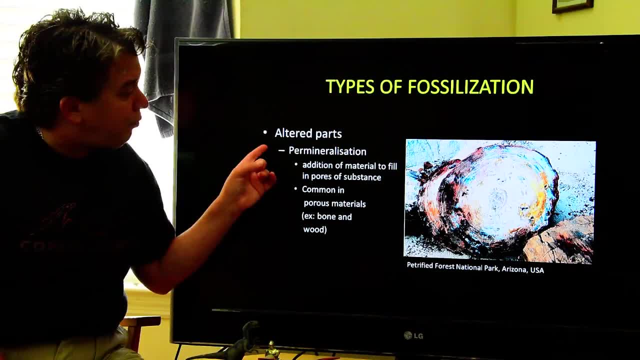 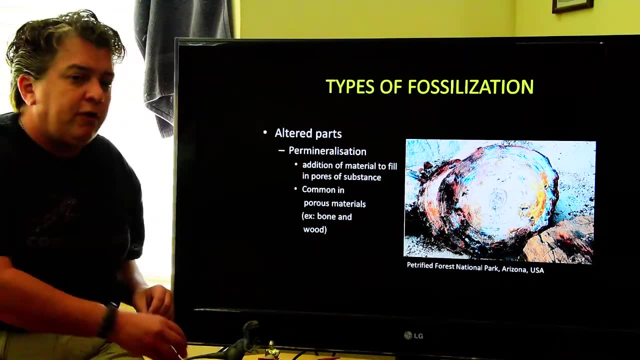 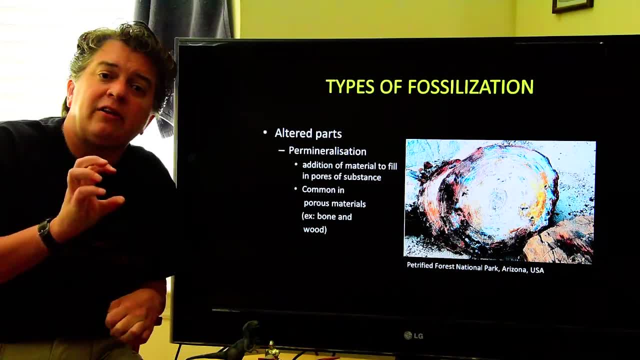 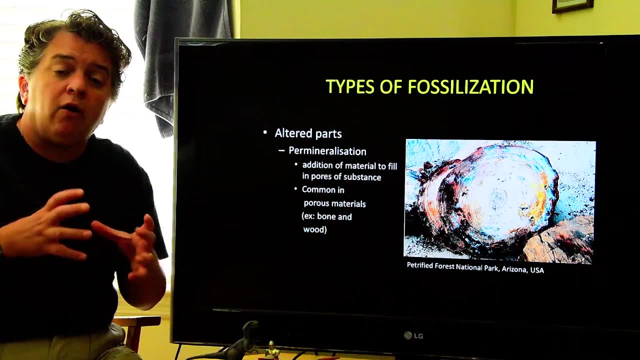 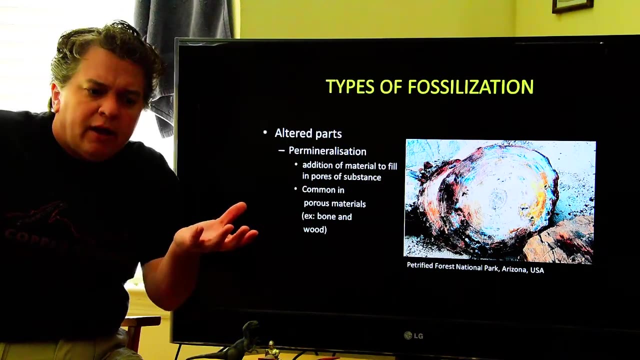 And there's two substances especially that have a lot of pore space in them. Wood is one of them, The other is bone, And so bone and wood often gets permineralized, because what happens is these groundwater can be flowing through the area where you're recrystallizing. 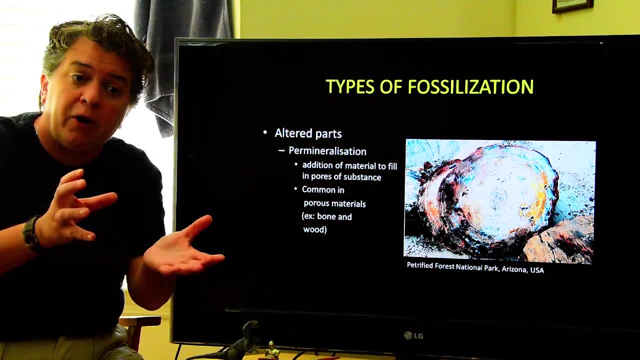 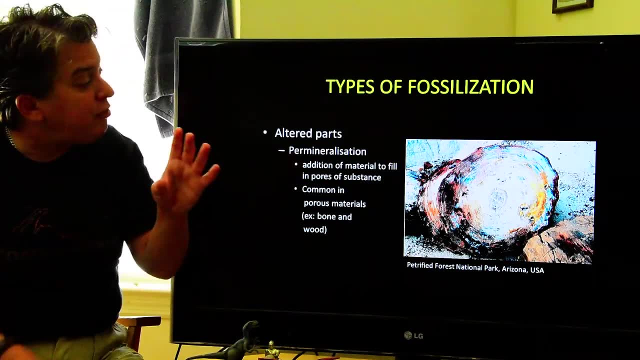 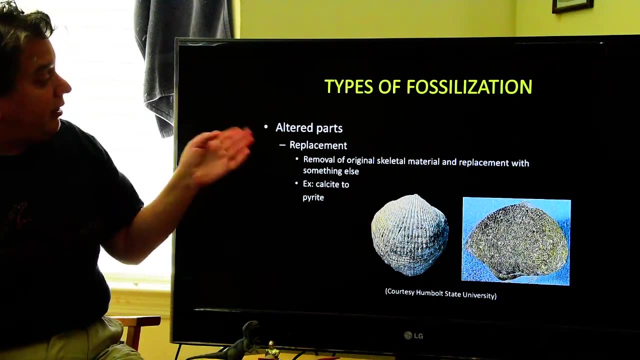 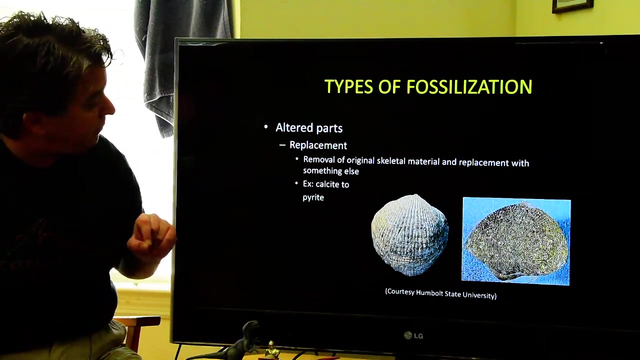 The area where your tree or your bones were buried, And the groundwater will then precipitate minerals in all of the pore spaces, thus preserving that fossil. Now, in addition to other types of altered parts, you can have replacement. Replacement is where the original skeletal material gets removed. 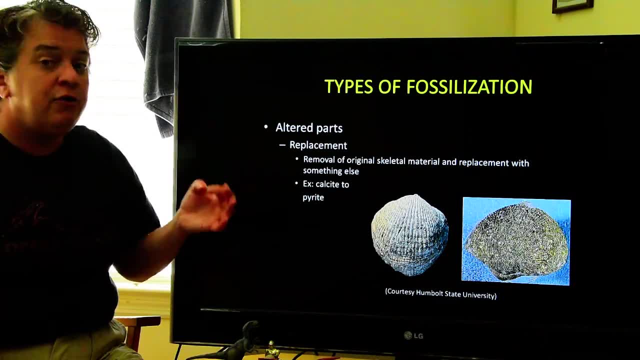 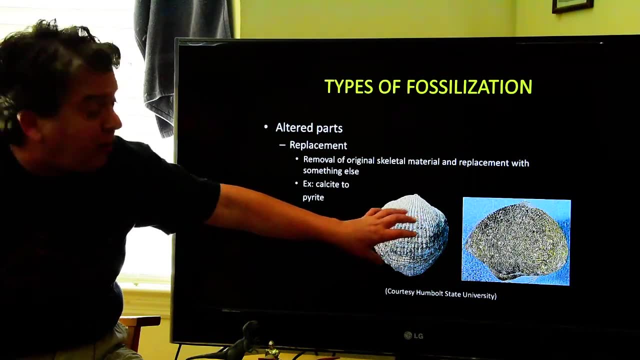 Replacement is where the original skeletal material gets removed. Replacement is where the original skeletal material gets removed And then a new mineral replaces it, And our example we have here. this is a type of organism called a brachiopod. It would originally have a calcite shell like this. 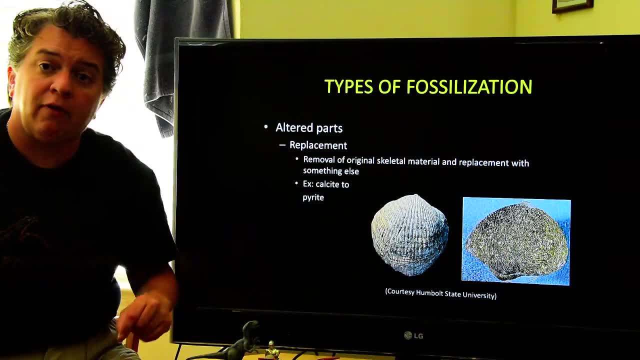 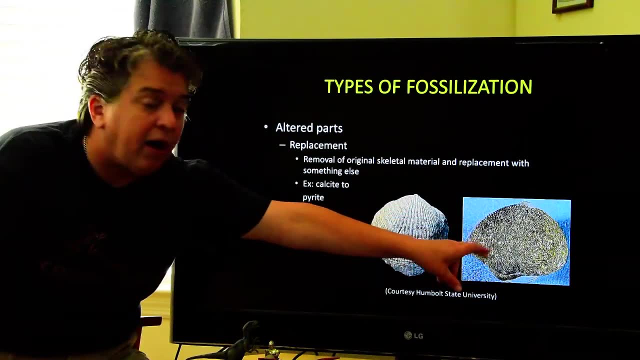 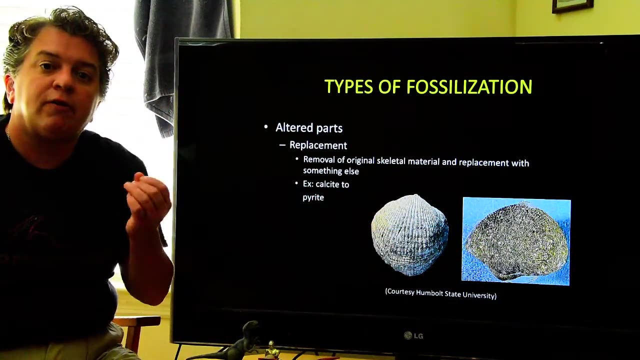 And in this one it's being replaced by the mineral pyrite. So totally different chemical composition. Calcite is calcium carbonate, Pyrite is iron sulfide. So we completely removed the original and replaced it with brachiopod And replaced it with a different mineral. 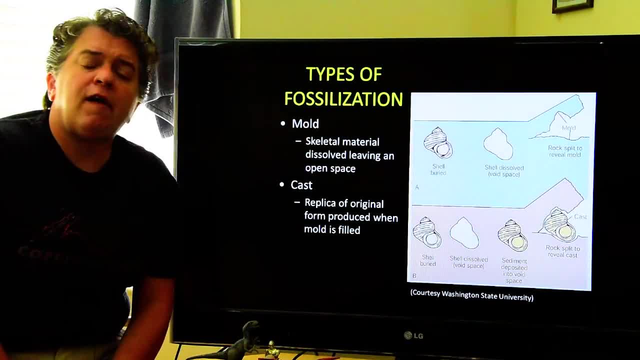 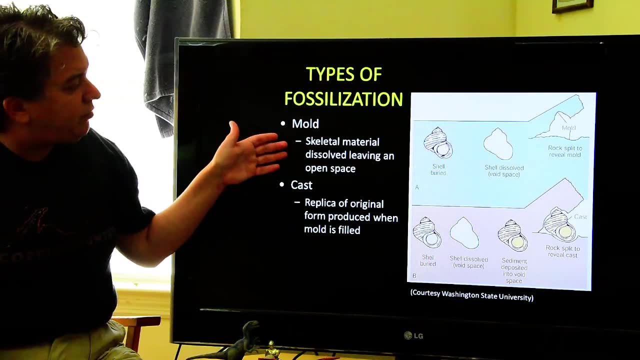 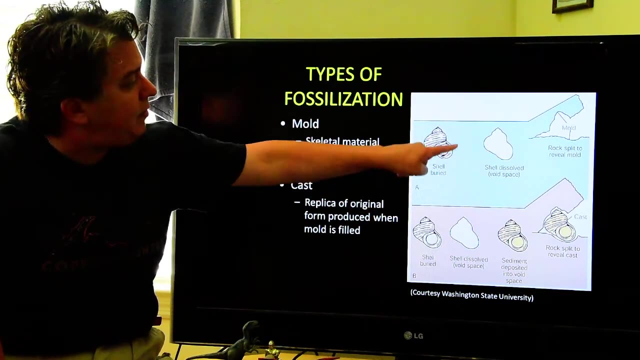 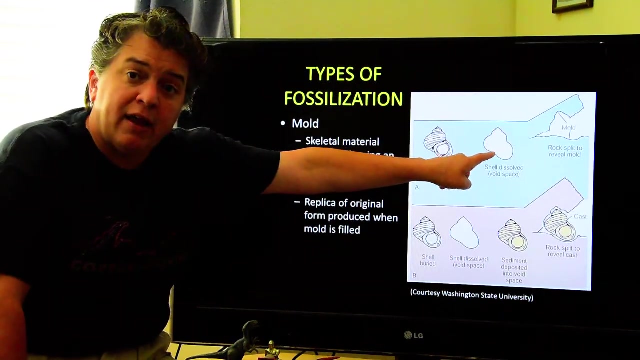 That's replacement, And then in fossilization you can have what are called molds and casts. So a mold is skeletal, material gets dissolved, leaving an open space. And that's what we see here in this top diagram. We have this shell gets buried and then it gets dissolved, leaving an open space in the 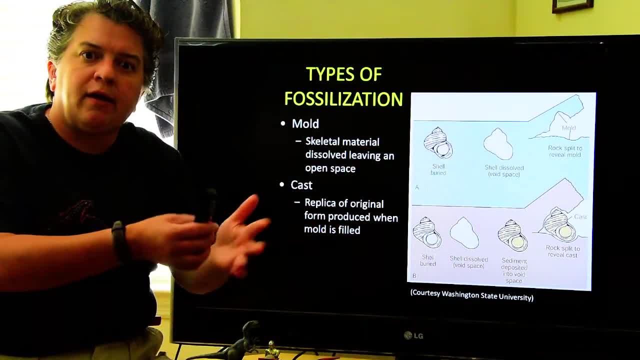 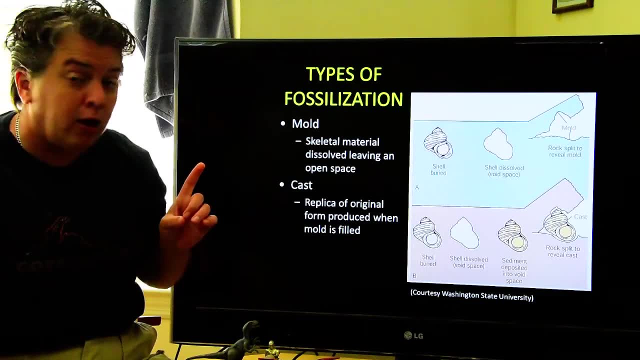 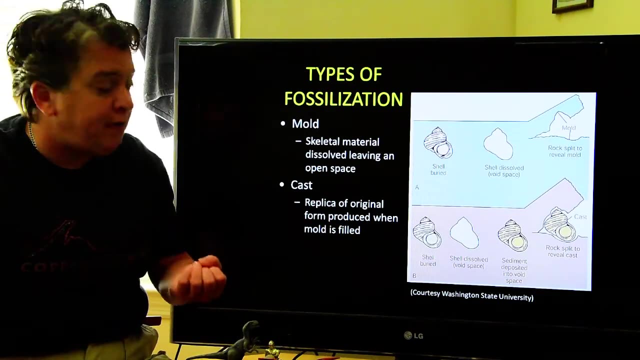 rock And we can then like, maybe when we're breaking the rock apart or so, we will end up finding that open space in the shape of that particular shell. Now, a cast is where we get a replica of the original when a mold gets filled. 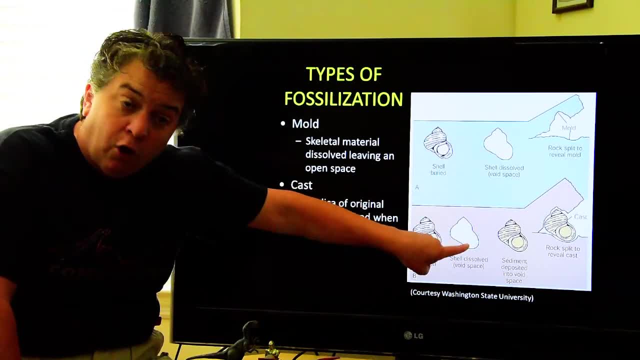 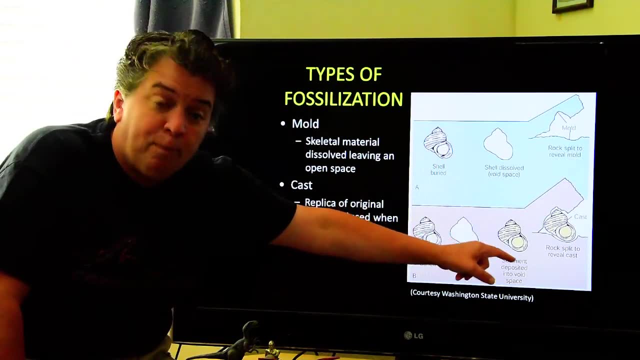 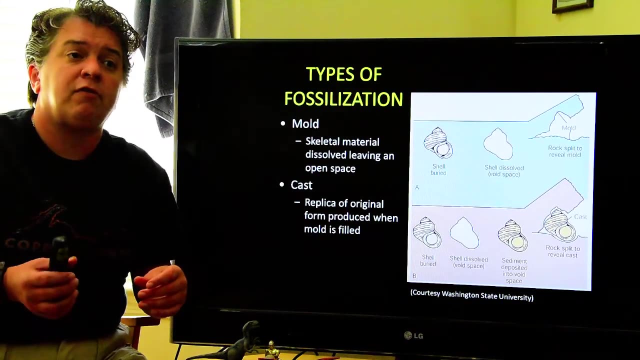 So we have the shell buried, it gets dissolved, we have this open space there, But then sediment or some other mineral will come in and fill up that open space and that's going to be the cast. It gives us a replica of the original fossil, but it is not the original fossil. 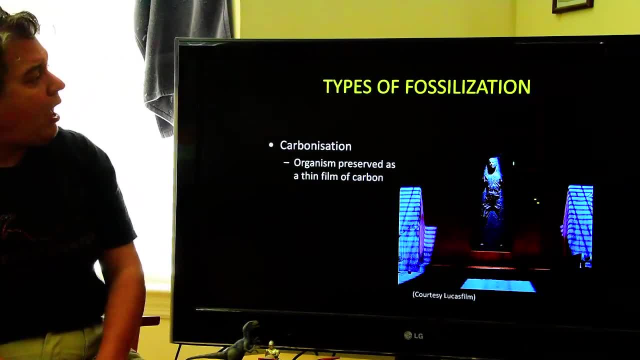 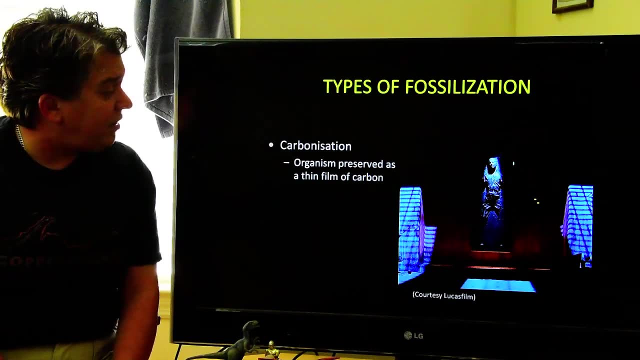 It's made out of some other substance. Then we also have carbonization, And carbonization is where the organism is preserved as a thin film of carbon, And I couldn't resist putting a little Star Wars reference in there. But really carbonization looks a lot like this. 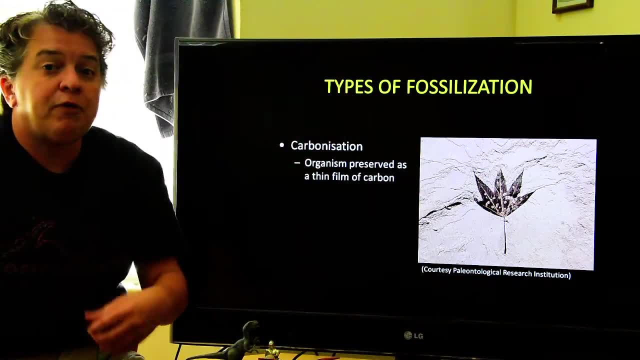 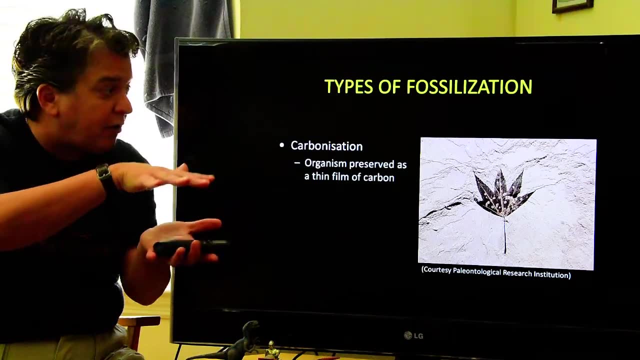 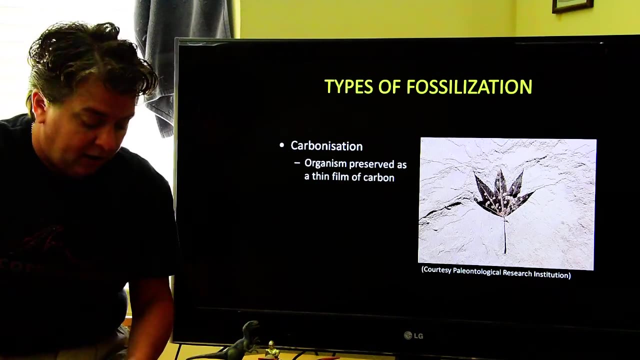 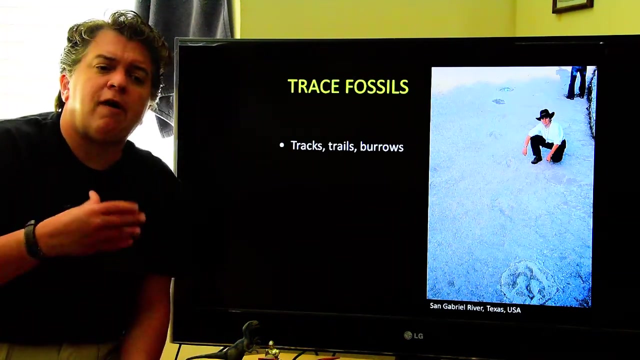 So here we had a leaf, and remember, organic material is made of a lot of carbon, and when that leaf got squished in between these layers of rock, basically it left this thin film of carbon showing us the remains of that organism. Now, all the previous types of fossilization were what we called body fossils. 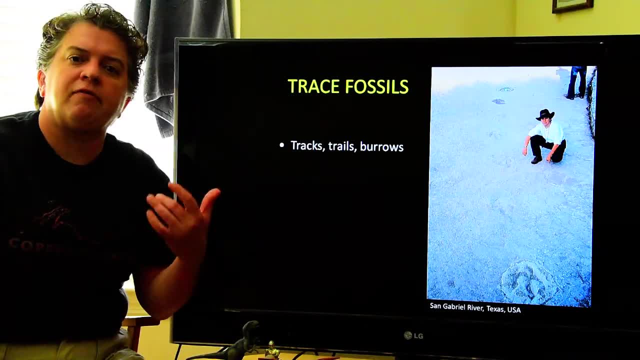 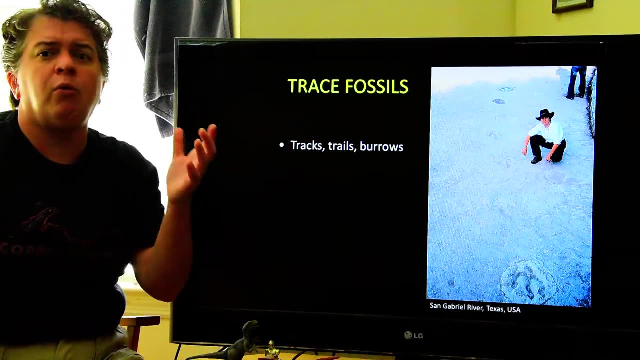 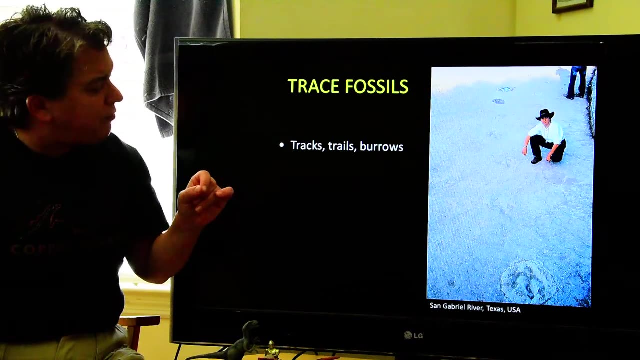 These are where some sort of actual piece of an organism is preserved. It was like an impression of the leaf, or it was a shell, or it was a bone or a tree trunk. We can also have what are called trace fossils. Trace fossils are indirect evidence of past life. 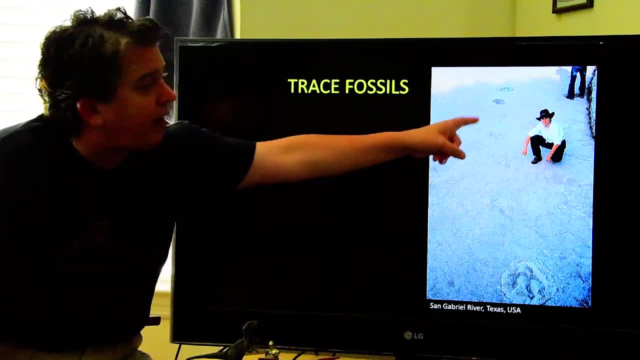 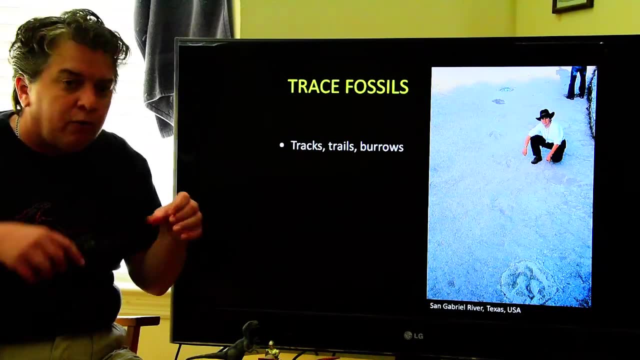 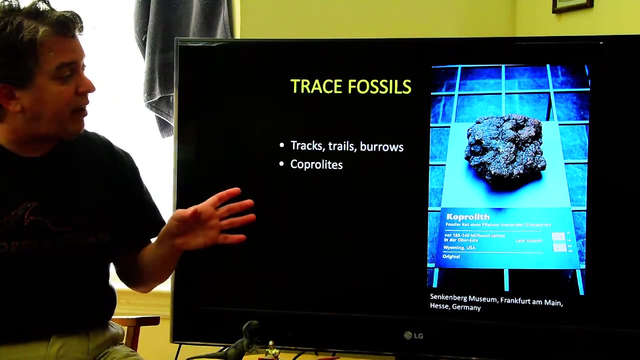 Things like tracks. We have this trackway of a dinosaur called Acrocanthosaurus, Trails that are left by organisms or places where they've burrowed into the ground. Those all count as trace fossils. Also, coprolites- Coprolites- are fossilized dung. 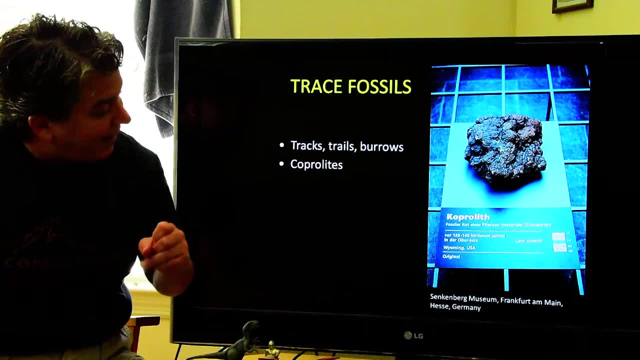 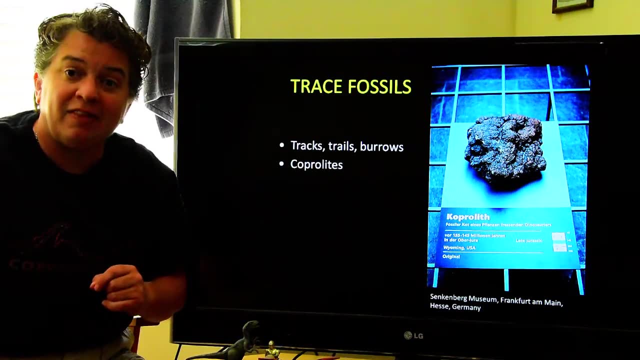 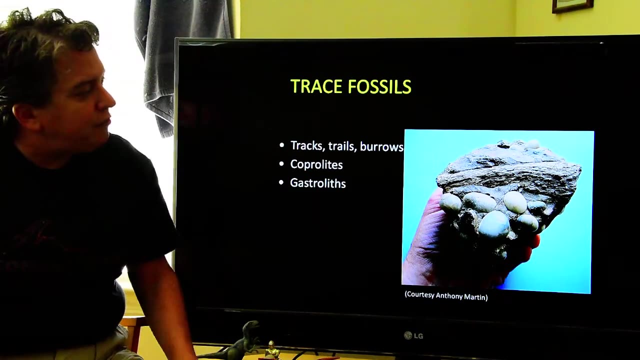 Fossilized poop. This is a coprolite of a plant eating dinosaur from the Jurassic. So it's not an actual piece of that organism, but it is definitely something that it left behind Trace. fossils can also be things like Gastroliths. 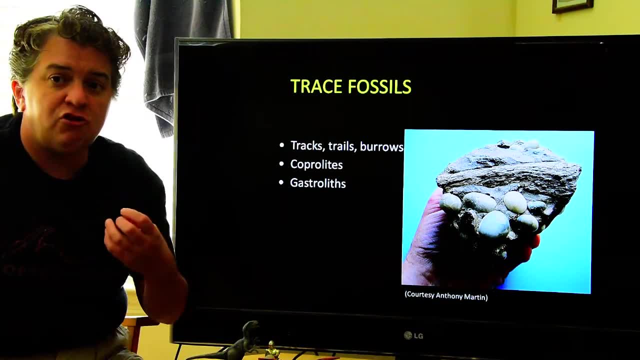 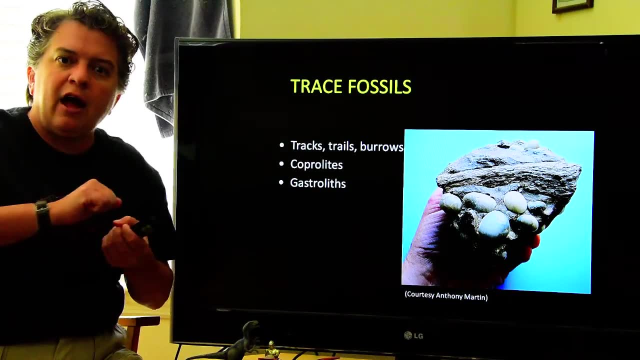 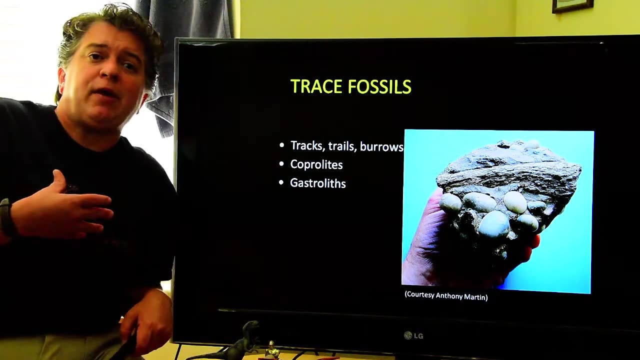 So some dinosaurs would actually ingest little rocks. Those rocks would sit in a stomach or a crop and help grind up the food. And that's what we're seeing right there. Those are gastroliths And they're not an actual piece of the organism, but it was a part of the organism, that it 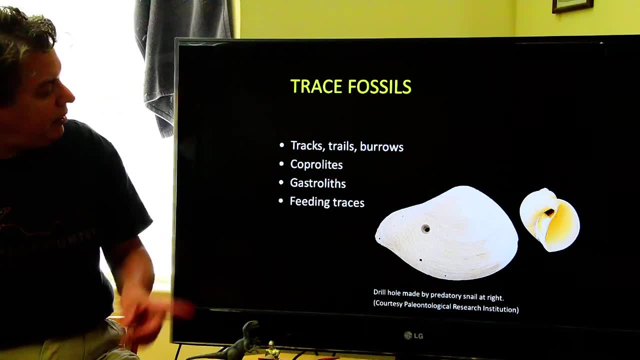 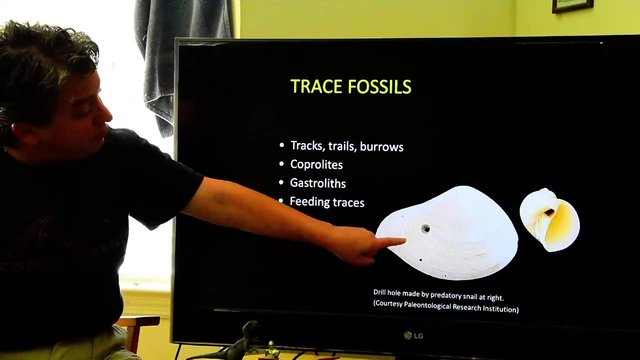 left behind. And then there are feces. They're eating traces. So we have these shells right here. And then we have this: That is a drill hole made by a predatory snail. That's the shell of the predatory snail. 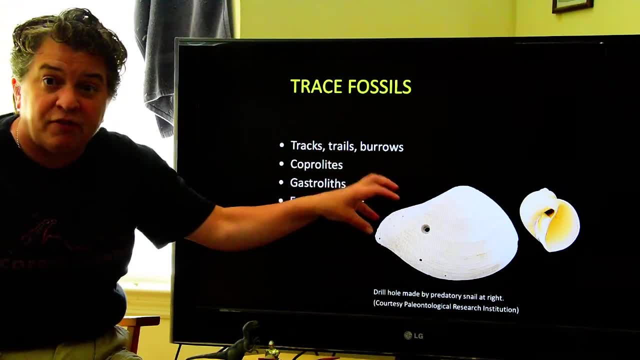 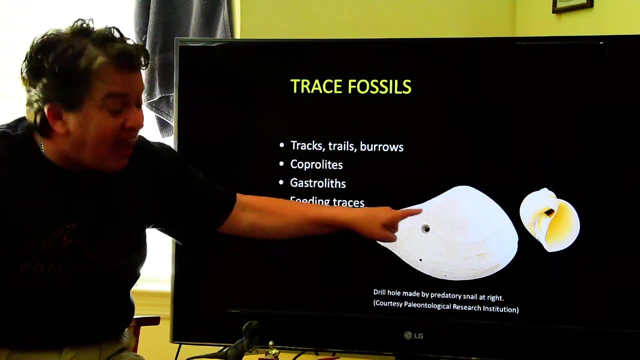 Comes up to this organism, It drills a hole in there and then it eats the organism, And so, even though the snail didn't leave a piece of its body there, it left evidence of itself there, And that counts as a trace fossil. 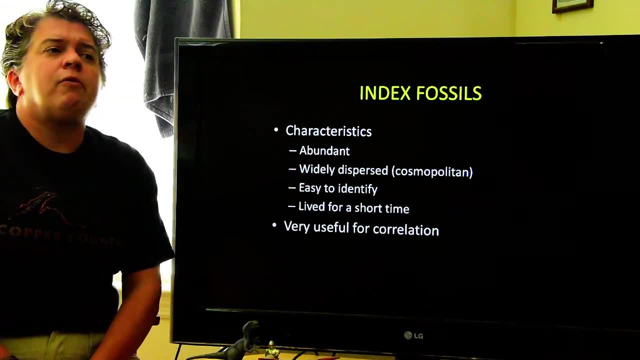 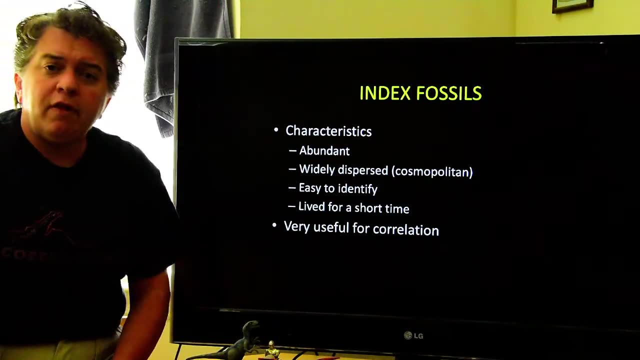 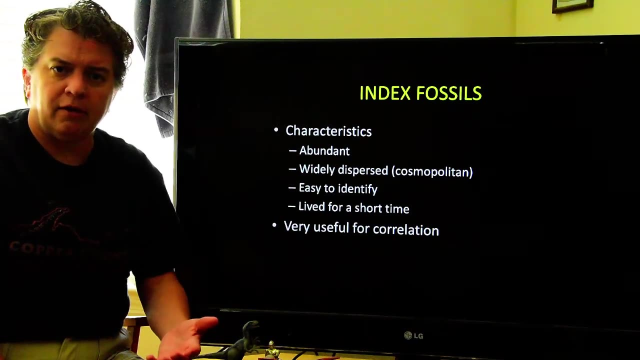 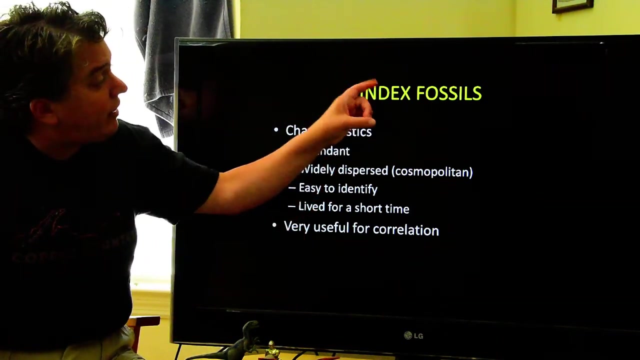 All right. so now we've seen how fossils can be preserved in many, many different ways, And one of the things that's very important in historical geology is figuring out when things happened. We like to know the timing of things, And something that can help us with that are index fossils. 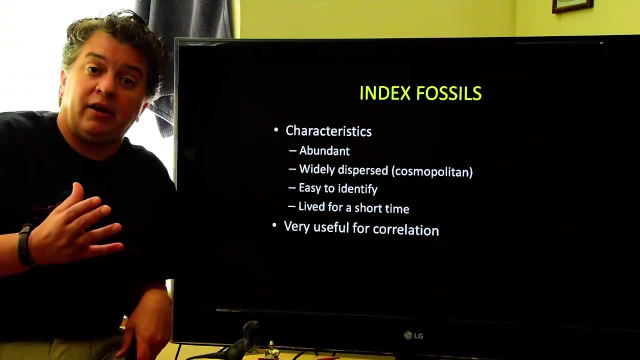 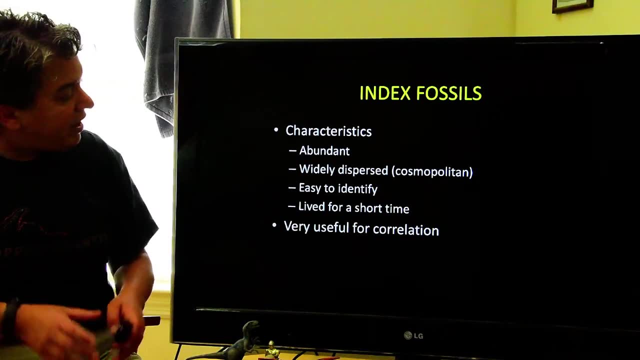 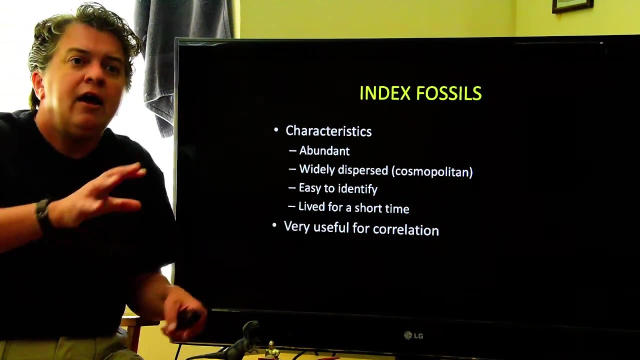 Index. fossils are organisms that were abundant, They're cosmopolitan, They lived all over the place, They're easy to identify And they only lived for a short time. So it's a certain species that only lived for this short time period. So wherever we find that species in the world, when we find it, we know we are looking at. 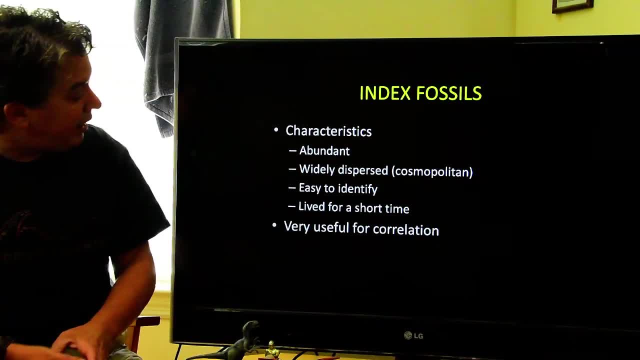 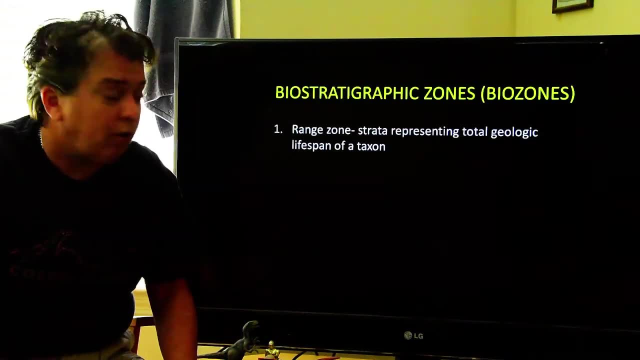 rocks from that specific time, And so this can be very useful when we're correlating rocks from different places So we can have a better understanding of the time. Okay, from different parts of the world, Alright, so in this concept of using fossils, 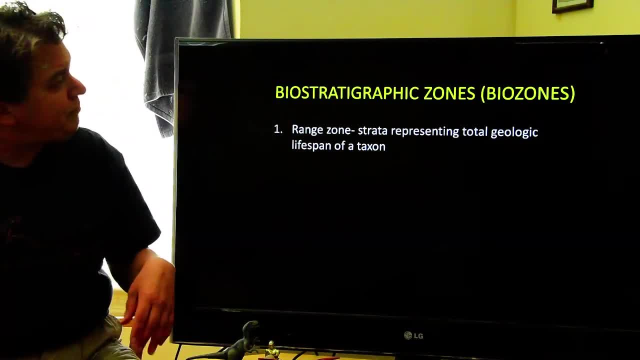 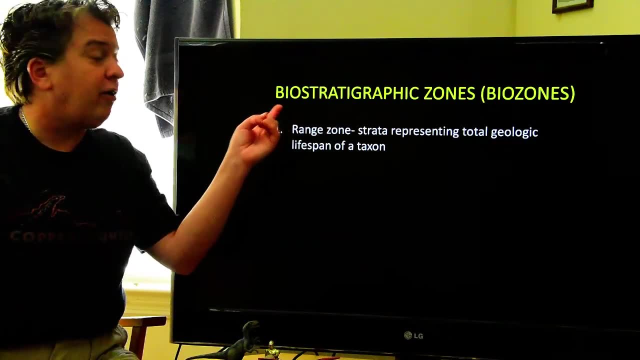 to help figure out when things happen, we have to know a little bit about what's called biostratigraphy or biozones. Well, bio means life and you know, stratigraphy is looking at the layers of rock. so biostratigraphy? 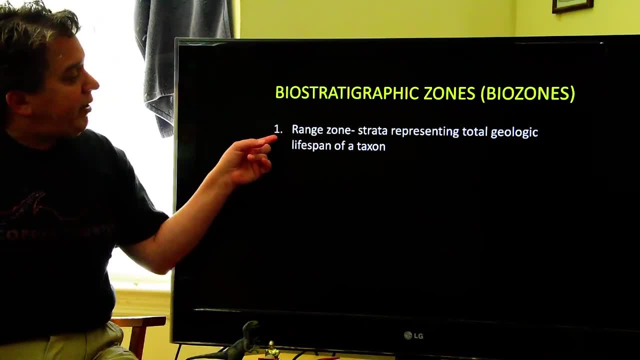 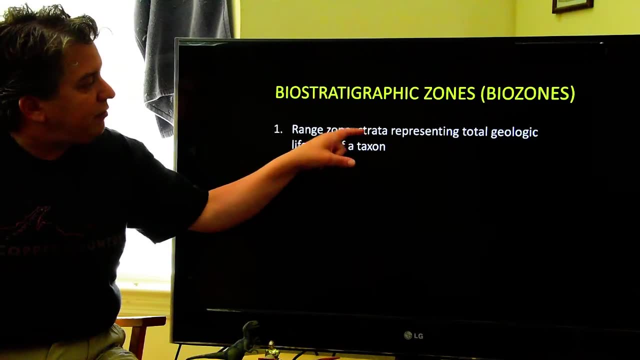 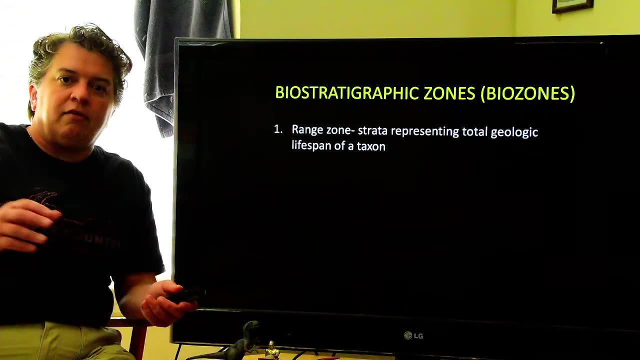 is looking at the life in the layers of rock And we can have what's called a range zone and these are strata, and remember, strata just means layers of rock. These are the layers of rock representing total geologic lifespan of a taxon, And a taxon is well. 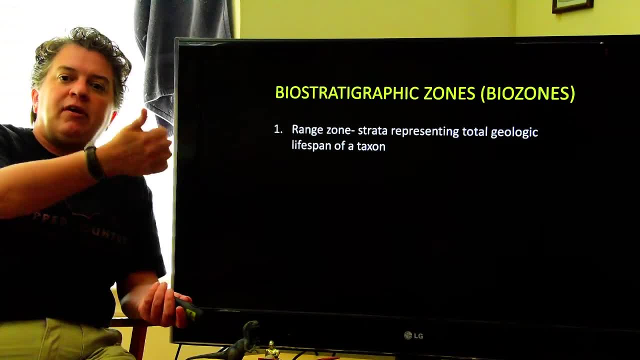 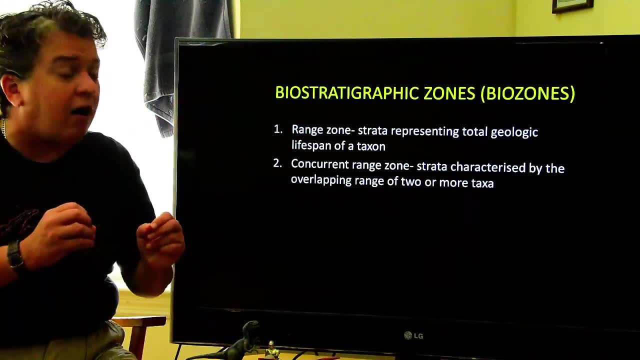 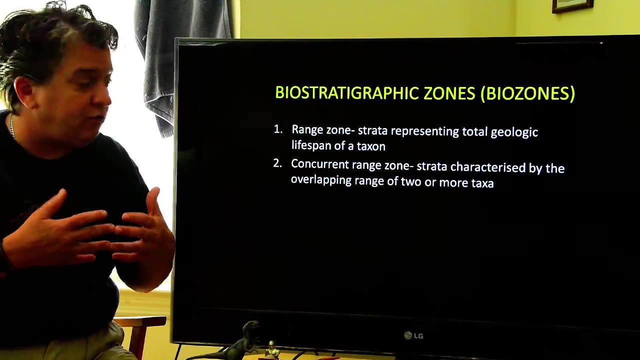 any group of organisms, so it might be a genus or a species of organisms. And then we also have the concept of what's called a concurrent range zone. These are the layers of rock characterized by the overlapping range of two or more taxa. So 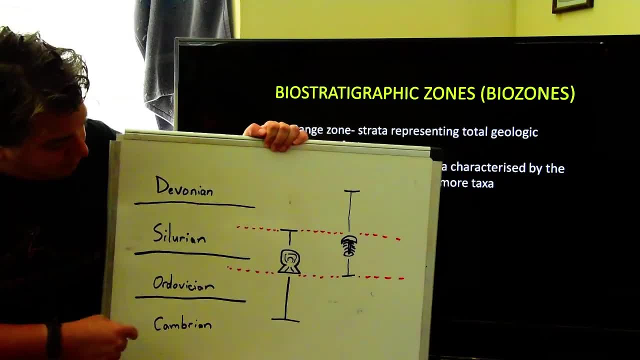 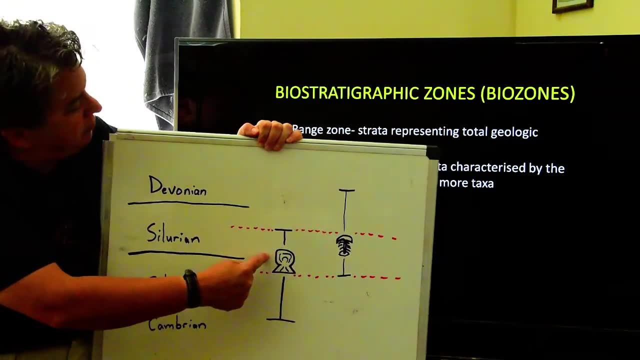 what I have right here. let's say: here's my time periods right: Cambrian, Ordovacean, Silurian, so on. Let's say I have one fossil right here. That's its range zone. It shows up here: 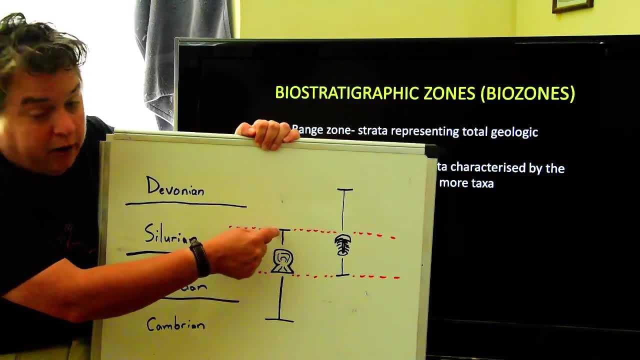 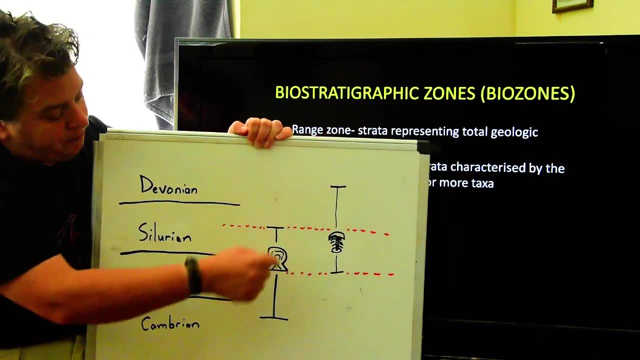 and that organism, that species, lives all the way to up here Or over here. this is a different fossil. it shows up there and that species lives all the way to there. So this whole time period is the range zone of that fossil. 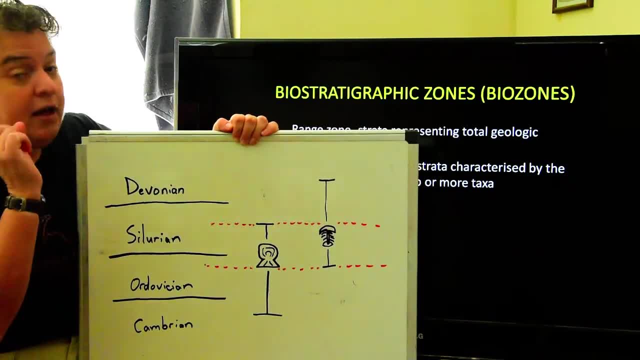 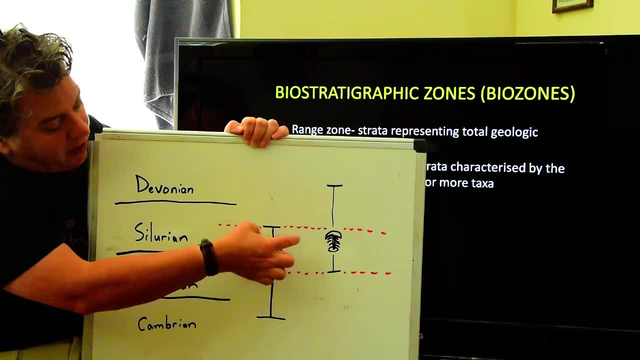 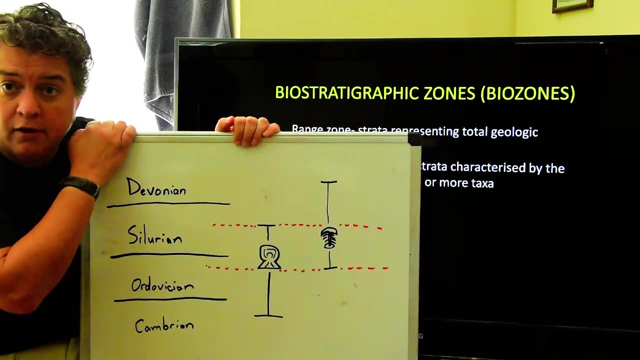 or this whole time period is the range zone of that one. The concurrent range zone is between these red dotted lines. right, because that's where those two fossils, that's the time period during which those two coexisted, And so we can then 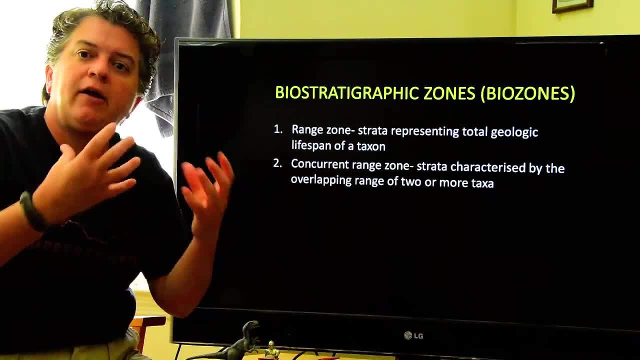 look at things like that: seeing where, if we find a rock with multiple fossils in it. and then we can look at things like that, seeing where, if we find a rock with multiple fossils in it, we can figure out when did all of those? 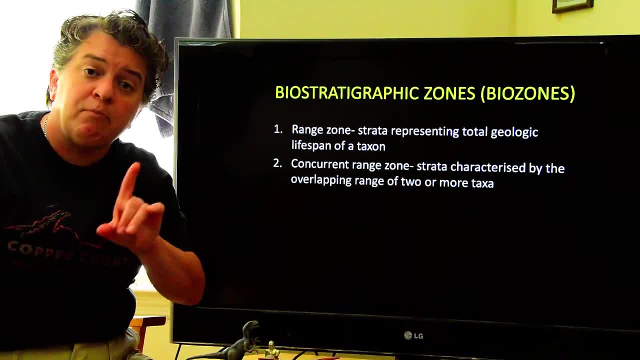 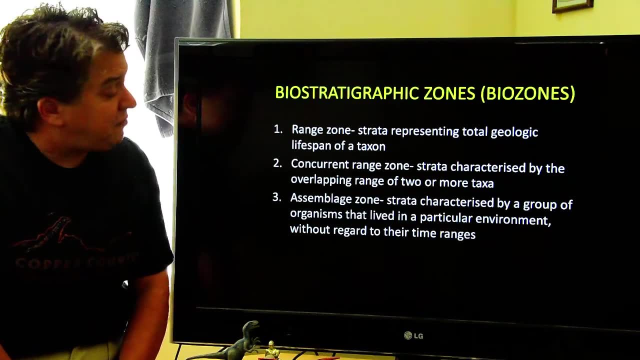 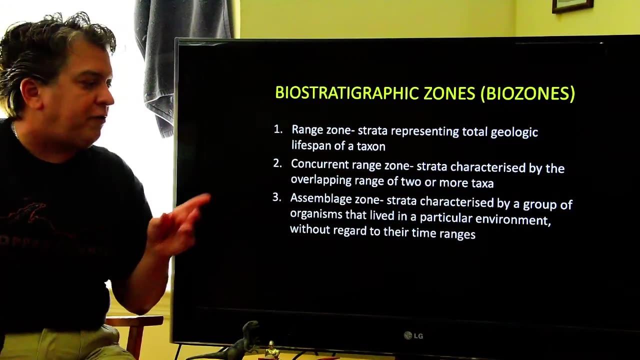 organisms coexist, and that must be when our rock was created. You'll also sometimes see something called an assemblage zone, and these are rock layers characterized by a group of organisms that lived in a particular environment. This doesn't really pay attention to time ranges. 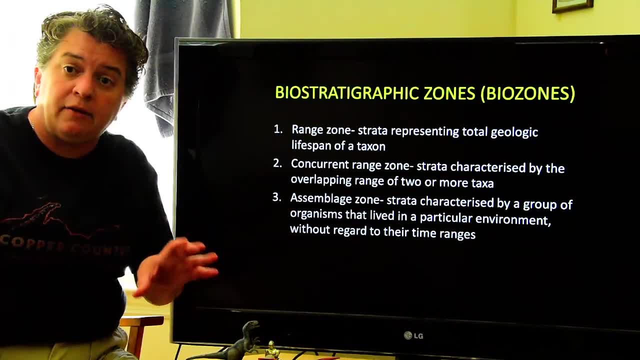 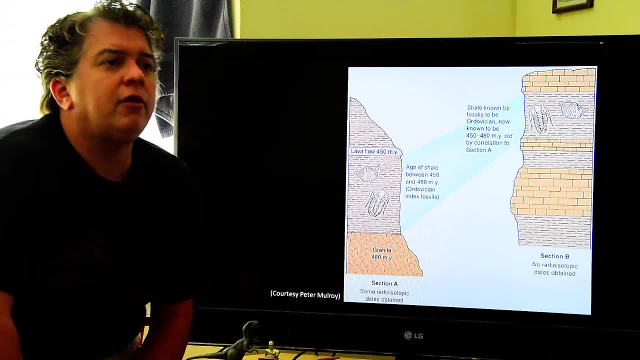 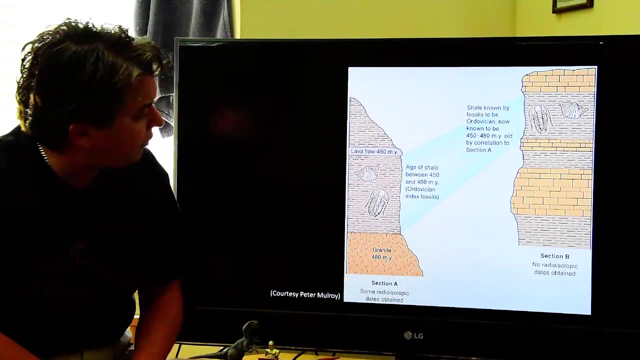 and I just wanted to put that in there because you might see that in your book and I just want you to be aware of what that is. So how can we ultimately use fossils and mesh that together with numerical dating to figure out when things occurred? 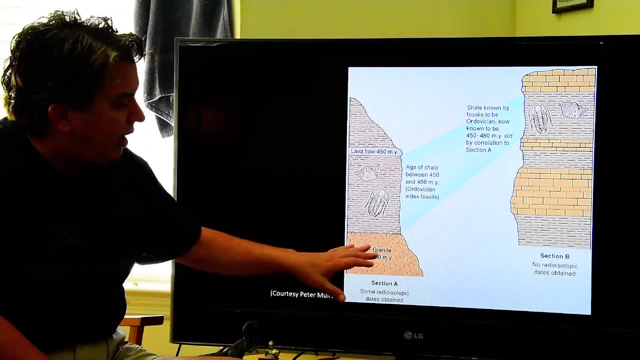 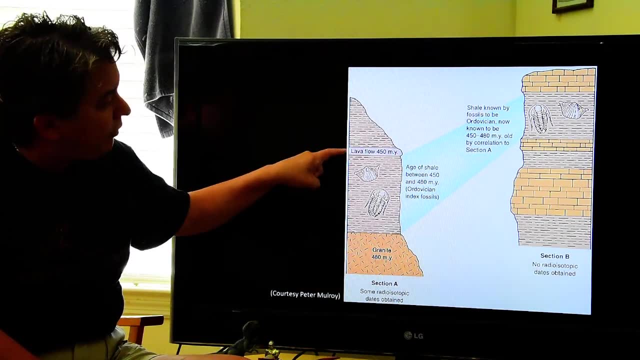 Well, let's say over here, this is my stratigraphic section, and I'm lucky enough at this section to have granite that's dated at 480 million years old and a lava flow dated to 450 million years old. And right here I have. 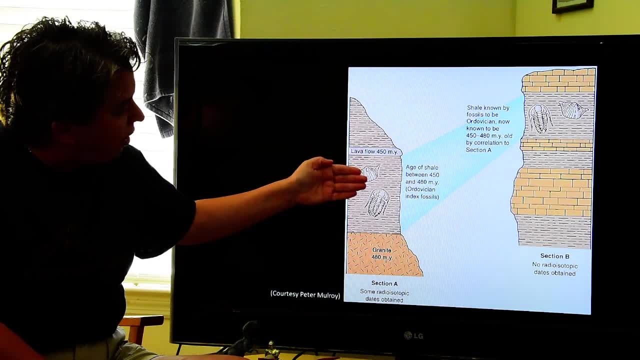 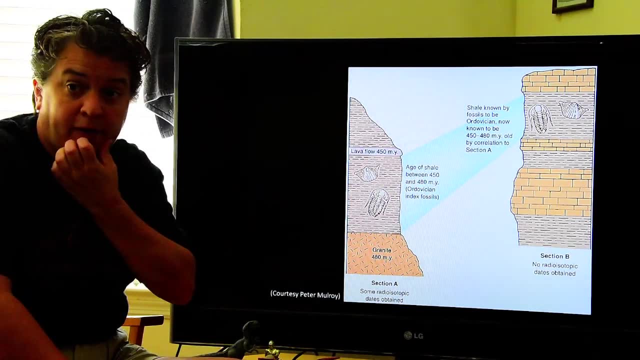 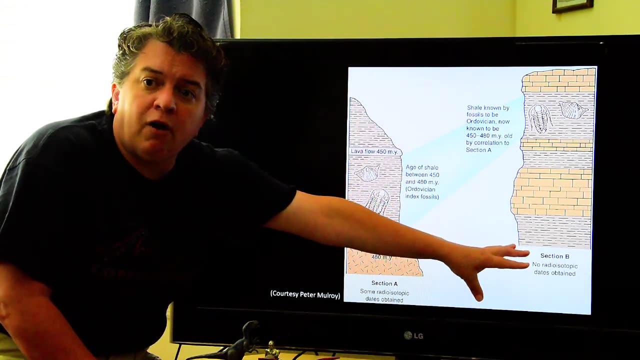 these two species. Well, I know, since that rock is between those two, it must be the age of that, between 450 and 480 million years old. Then if I go over here- over here I have no igneous rocks- that I can get the numerical. 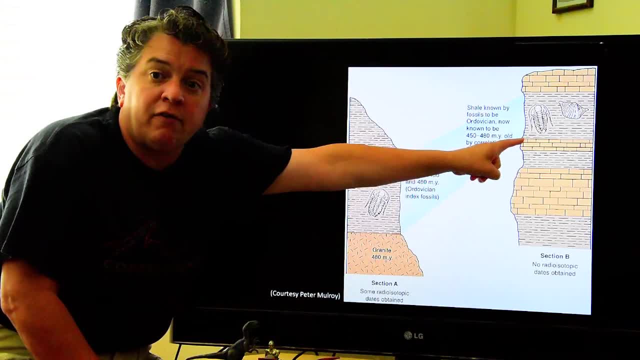 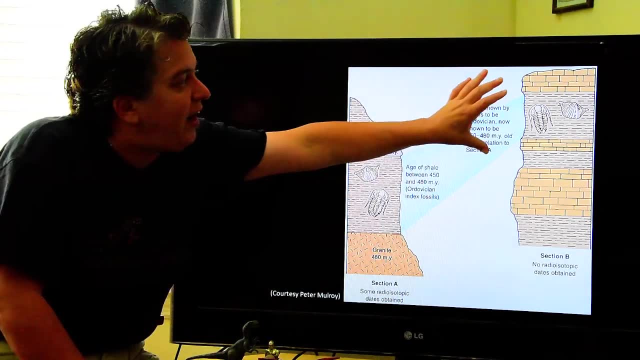 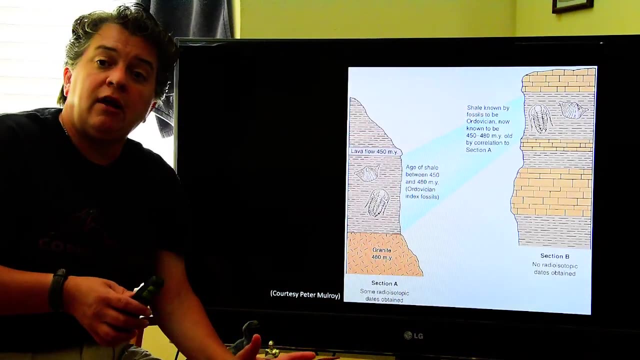 ages on, but I have those fossils and I know those fossils lived between 450 and 480 million years, So I have a good idea that that rock formed in that time period. So you can actually put together numerical dates and some of your index fossils. 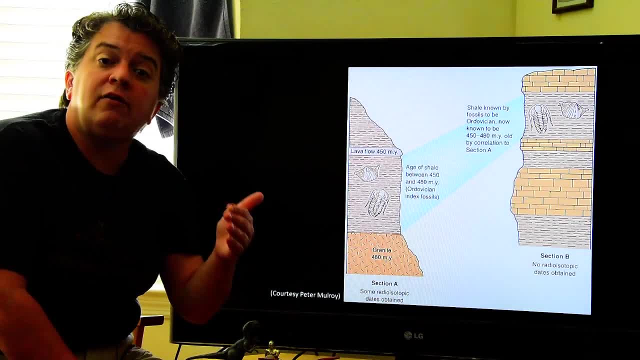 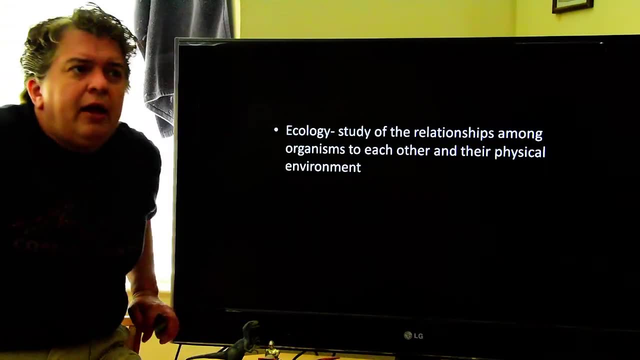 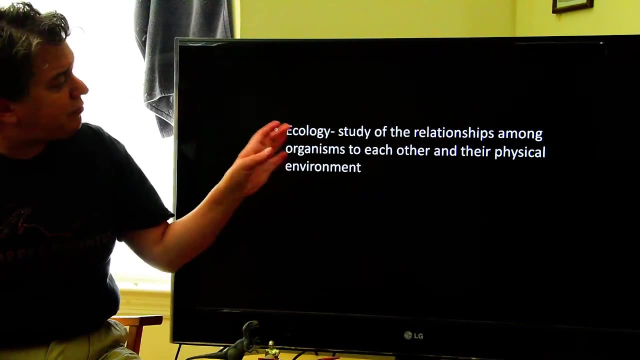 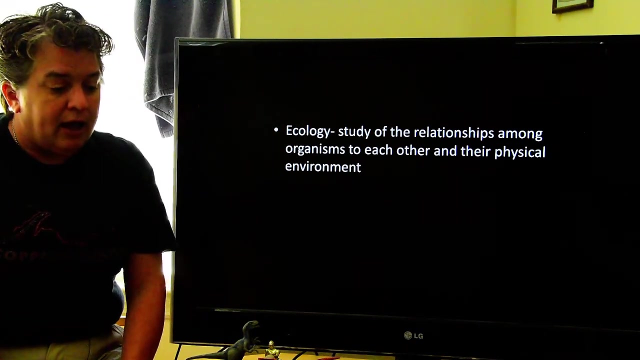 to get a nice view of when different events happened on earth. Alright, so a part of studying biology is called ecology, And ecology is of relationships among organisms to each other and to their physical environment. And in historical geology we spend a bit of time studying paleoecology- right ancient. 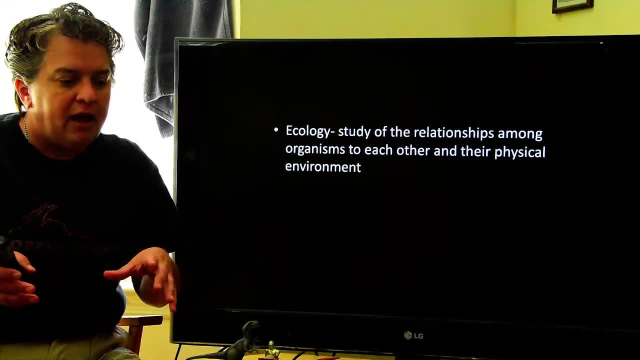 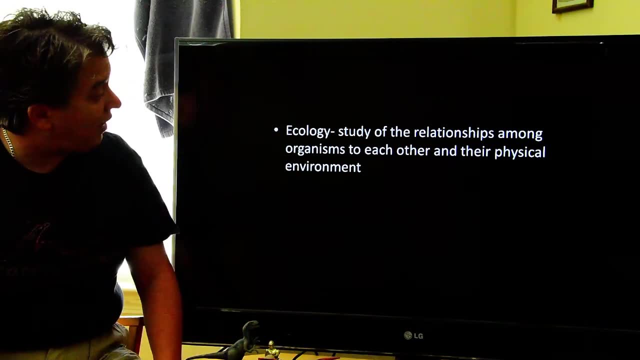 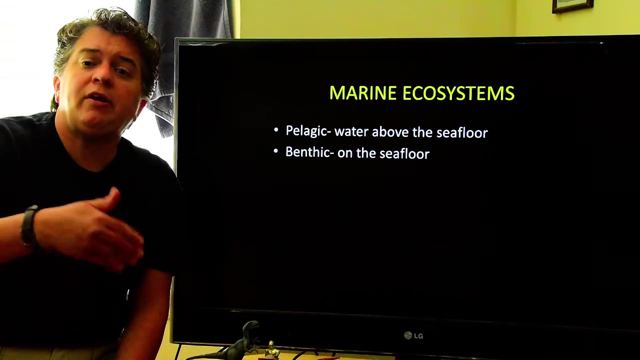 ecology, because we get all of these different fossils and we can then start taking a look at how those organisms related to each other and what their environment was like. So I'm going to introduce some concepts of ecosystems that we will be talking about throughout the semester. 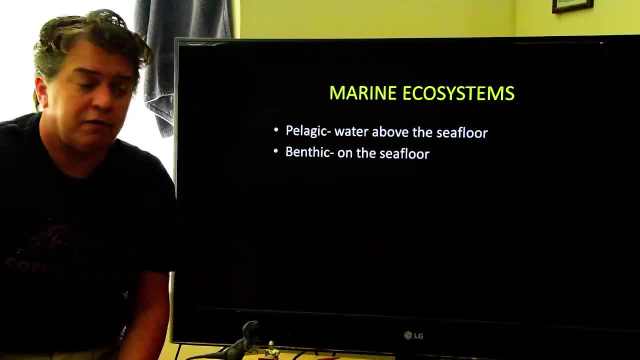 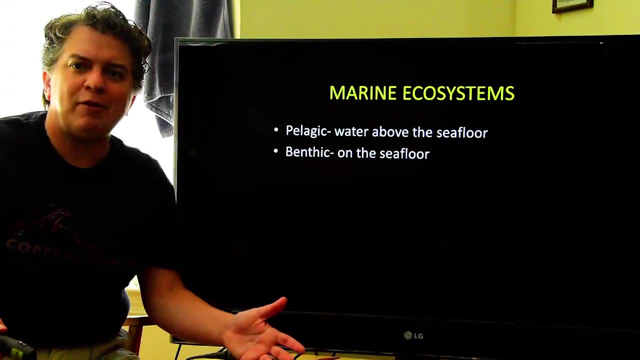 And today I'm going to be introducing marine ecosystems. And when I do this today? because, hey, Earth has, like what? 70% of the planet is covered by water, so we've got a lot of rocks that were created in water.